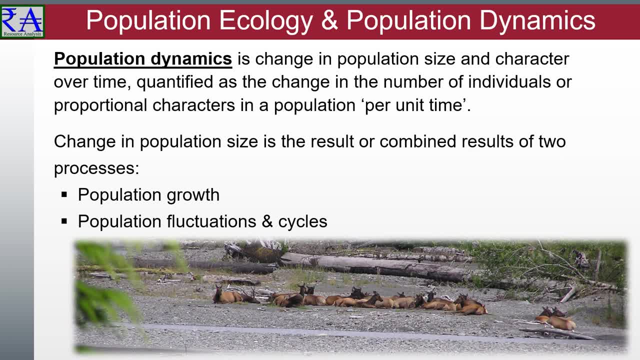 and I'm going to show you the salmon. And this is the salmon that we saw on the video. So, as we looked at the salmon, why? Because they're eating everything around the riverside and that was shading to the river. But let me even back up a lot. If I go back to the statehood of Washington, originally there was expeditions going from Seattle over to the coast to meet with the tribes. It was part of the time when the tribes got their treaties in 1850. there was a lot of delegations going over to the coast and the way they got there they couldn't 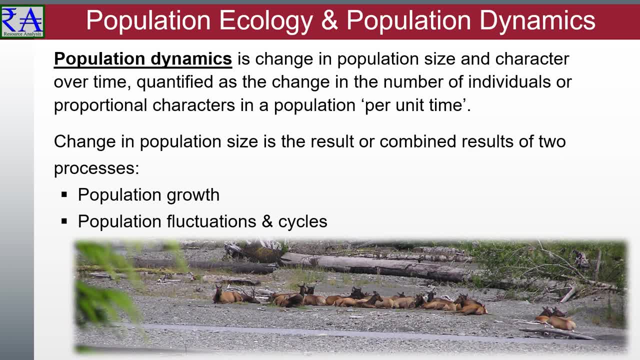 drive 101. There was no Olympic loop highway. They had to go over the mountains, They had to come down into the river and progress down to Lake Quinault and then down to Tohola to meet with the tribal councils. How did they get there? Well, they used the rivers Very tough, As they wrote in their 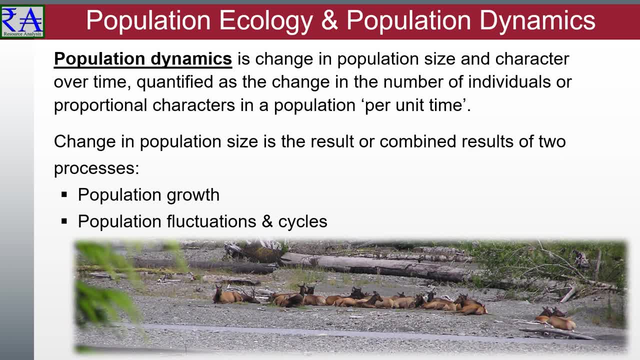 journals. they could not traverse those rivers. They were plaque full trees crossing the river. They had brush and debris piled up deep. It was unnavigable by the people on the boats. There was a natural balance of the ecosystem. The wolves were there, The elk were there, The deer 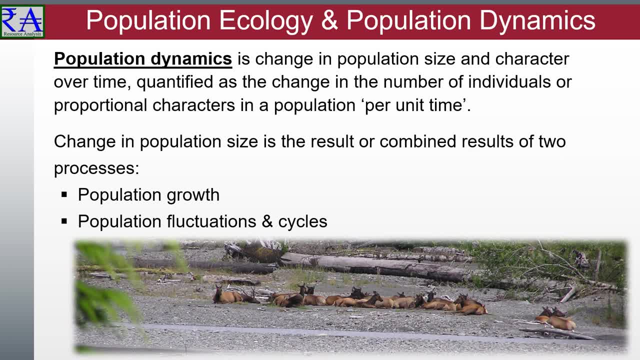 But that built up that cover for the river that was shading. There's a lot of nutrients being cycled into that river system and that helped the salmon, That helped everything else down the line all the way to the poor point of the littoral zone going out at Tohola of the razor clams. 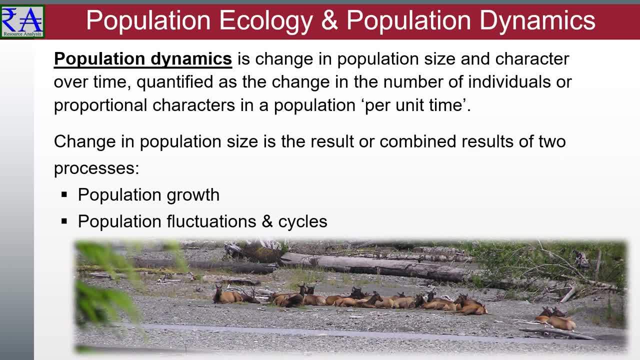 the starfish, the mussels, Every other critter that relied on high nutrient levels coming out of that river into the food source flowing out into the ocean. We messed it up, didn't we? That's the interconnected level that I'm talking about throughout this population dynamics talk. 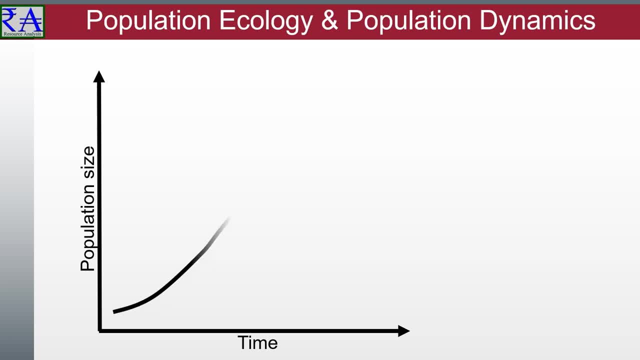 Because what we're going to do is start to look at this growth of the population. It can be a growth of the individual. How does it peak, How does it trough, How does it go up and down? Is there a level of equilibrium in that graph? Well, obviously, that straight horizontal line is the 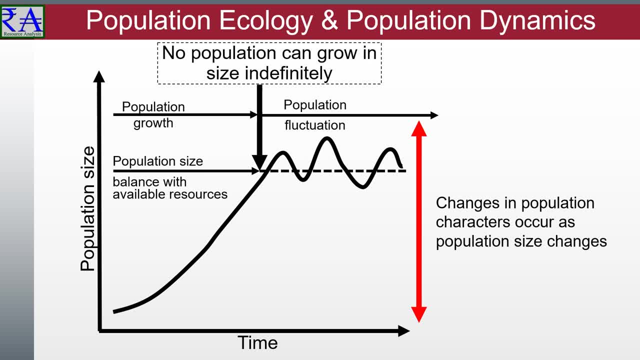 equilibrium level. That's the level of equilibrium in that graph. That's the level of equilibrium in that graph. That is what the population in that environment can be sustained at. There's a period of time where it's growing super fast and then the growth starts to slow down and it peaks out. 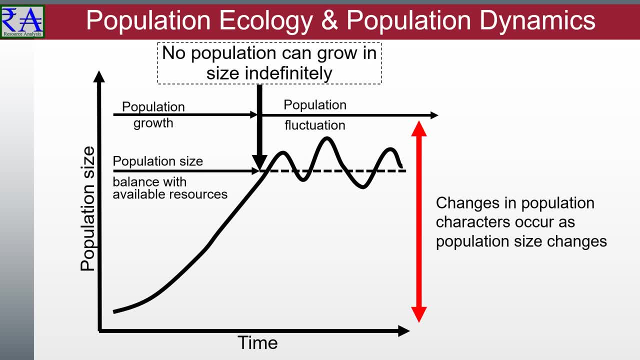 Maybe it peaks troughs, peaks, troughs. That's just a normal level of that population dynamics and we're going to use that as a way to express the carrying capacity of an environment. I didn't say of a forest, I didn't say of a lake, but you can apply this to just about any ecosystem where. 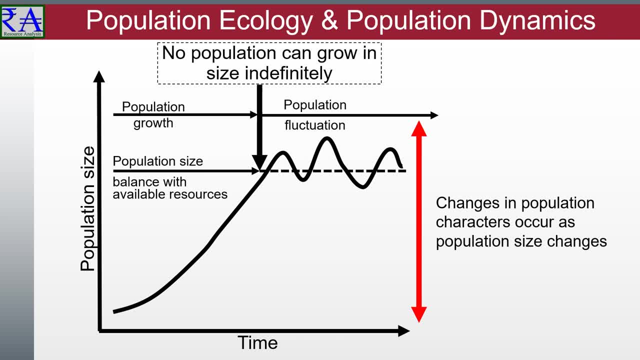 you have different species living. Well, we got to look at what can that environment support? Super simple on that respect that we can say, yeah, we see how that goes up and down. but the double tough thing to do is to look at these. 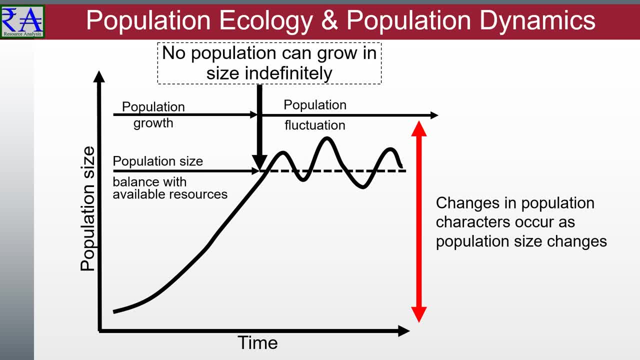 species' equilibrium models and predict it. And we're humans, We love to predict things Right. Everybody is looking at their grade at mid term to know what is their grade at the final going to be. Is that a predictor? Well, obviously it's an indicator. Can you predict with one point? source. 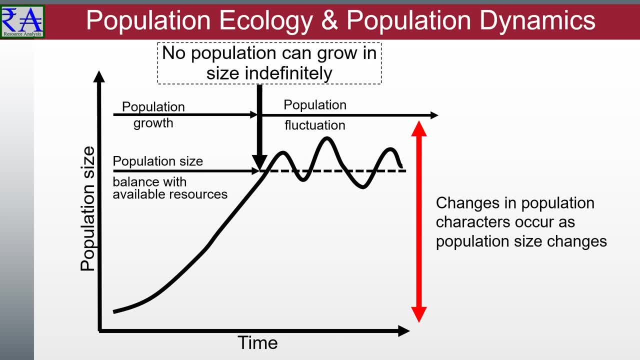 Probably not Right, Right, Okay, as you can, in terms of the natural environment, to predict how many critters it can support. That may be elk. Well, the elk populations- I talked on that just a moment ago. again, What is the number of elk that can be supported? 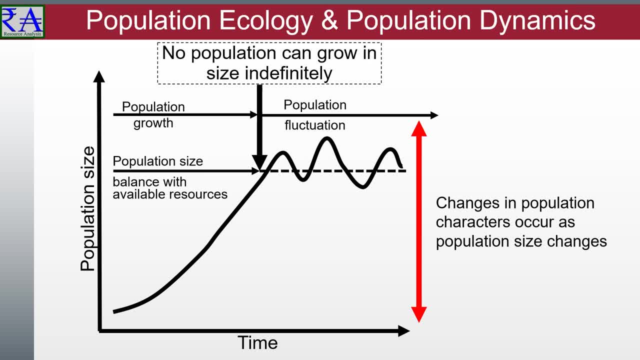 on the Olympic Peninsula. Well, you gotta ask a very obvious question: Depends. do you have wolves, Do you have an apex predator? Don't have the apex predator, then something else is gonna be the limiting factor. What could it be? 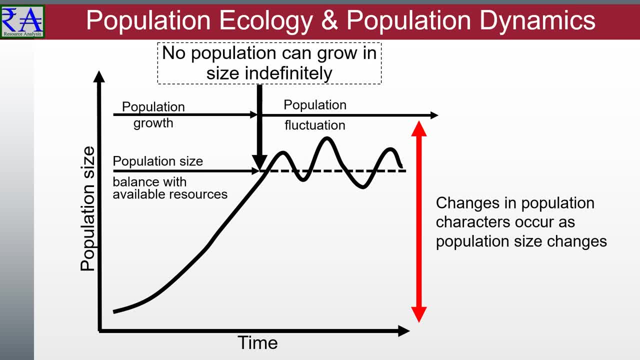 Elk do? they need space, They need food, They need water. Those are gonna be the limiting factors right there. And those elk in the previous photographs laying in the river they've shown that they can eat all the brush right up to the big conifers that they can't eat. 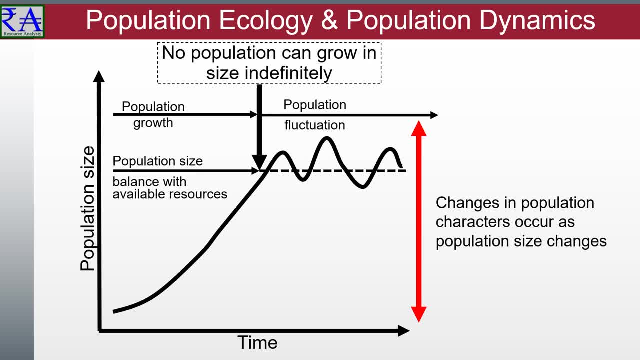 They'll eat them down. They'll keep eating them down, No matter how much rain you get, the plants can't keep ahead of them. That's gonna be a limiting factor for the food source for those elk, And that brings up a lot of questions now 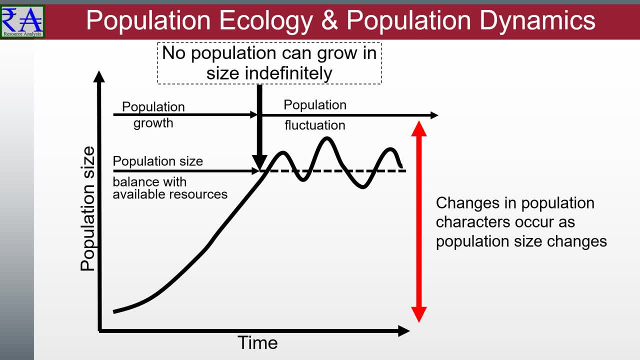 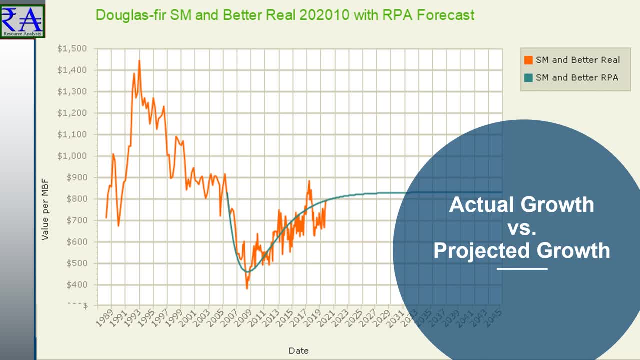 What are the limiting factors? That is something that we do with making those predictions, those forecasts. I'm a forester, I'm an ecologist, I'm also an economist. The graph you see right here is prices for delivered logs in western Washington. 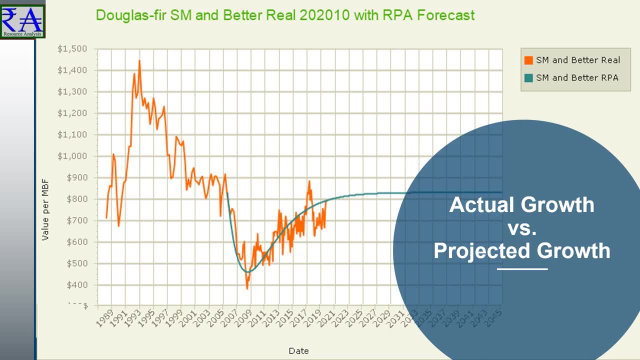 of a certain sort and grade. In this case, as Douglas Spurs, the sort, the grade is SM, and better that's sawmill and better It's a log that you cut out of the trees. I do a price prediction in real terms. 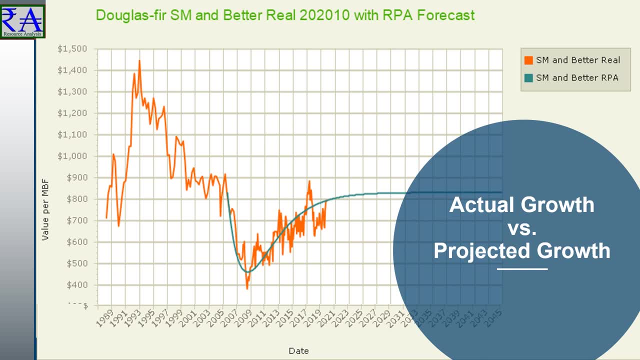 and the way I built this model was to look really back to ecology, exactly what I was just talking about: that period of time where you're having a peak and a trough or, in this case, a trough and then another peak. This was the Great Recession in 2009.. 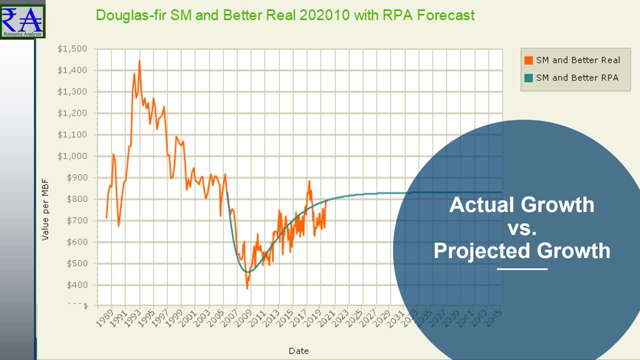 That Great Recession just tanked our economy and it tanked every industry within the economy. For all of you who've had some indication of something called the Markov Chain Random Walk, okay, this is a Markov Chain Random Walk theory with return to baseline levels. 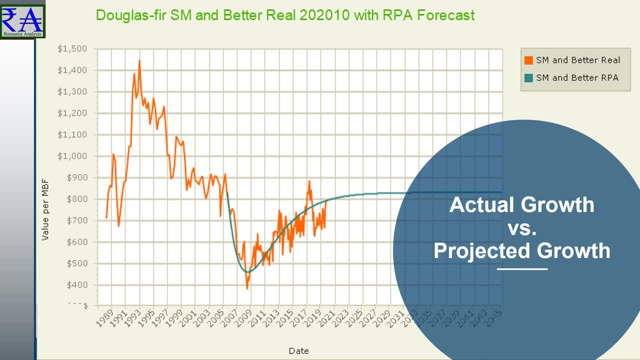 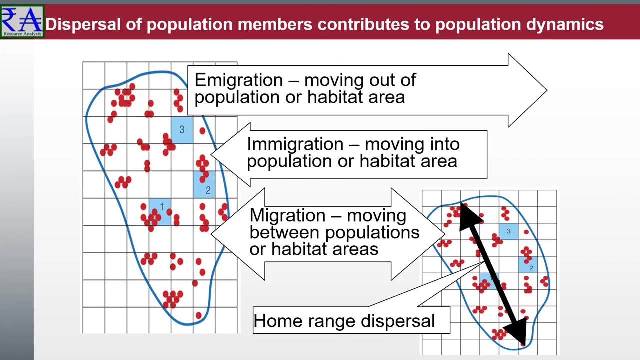 Found this not just because of the economic side of it, but because of the ecological side and how I applied that same kind of thinking and that philosophy to predicting species density and mass and distribution within a natural environment, And we can actually follow those along as we look at these questions. 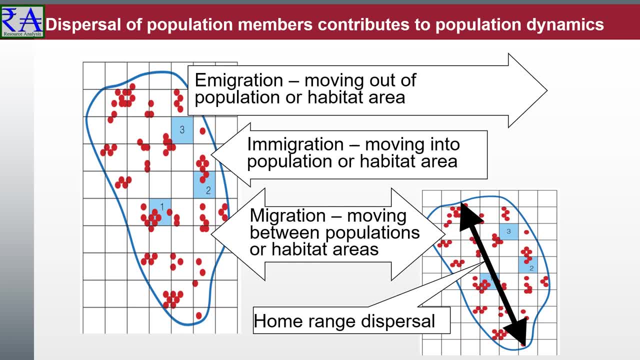 What is that home range? We saw this graph before Immigration. emigration and then natural movement of the species, like the video I showed you last Friday of 150 elk moving across Montana. single three, four, five, single file, we're gonna jump the fence. 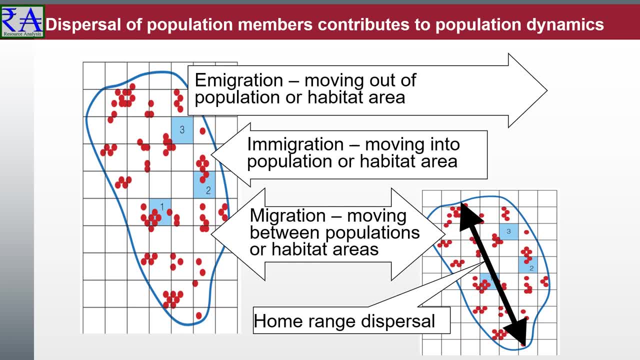 and go to our spring calving grounds. Okay, that is a natural movement of that population from one habitat to the next. It's not just one environment that they live in. In Montana they're moving a boat 50 miles one way. 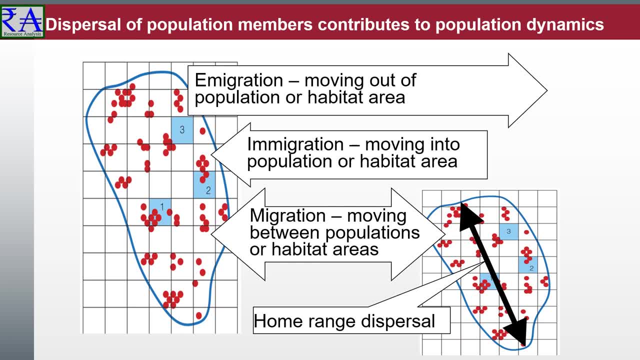 100 miles round trip. except they never go straight. They go in oval shapes, They're moving around. That's part of their species distribution model. because what is it gonna do? Tracking them, wanting to be able to predict how many elk am I gonna have? 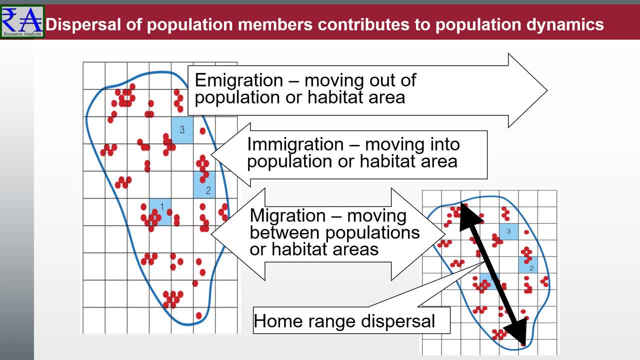 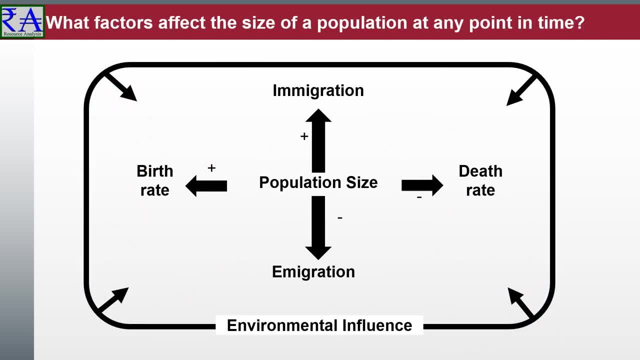 How many elk can be supported in that habitat that they're going to and coming from, That they're spending part of their life cycle in. That's a lot of big questions that are gonna touch onto things like birth rates, death rates. You're gonna look at carrying capacity of the environment. 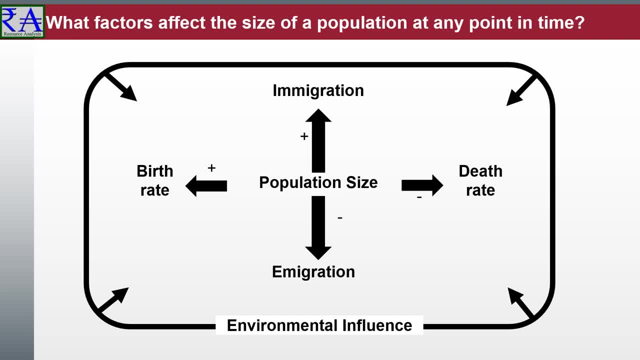 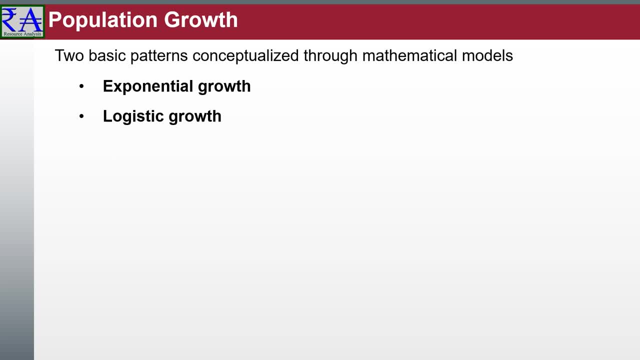 You just pick these things together and that's gonna lead to your estimate of what that population size is, And then we get to have the fun discussions about the different kinds of growth. What I'm gonna say is a lot of these growth, whether it's exponential growth, 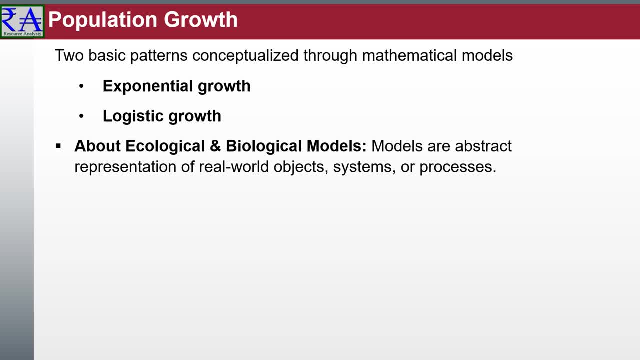 or logistical growth. they're gonna come in every population number increase. That's a mouthful right there, isn't it? That idea that initially they're gonna grow pretty fast, numbers are gonna get bigger, or the individuals are gonna get bigger if you're a tree. 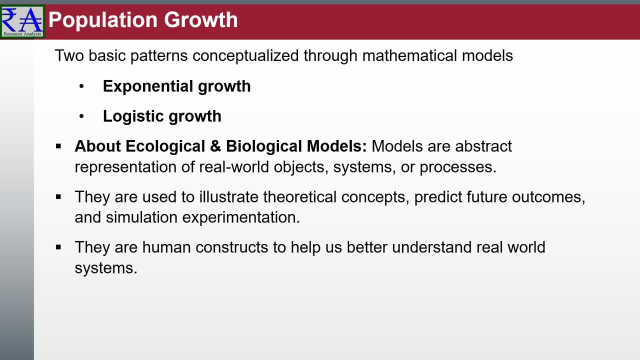 Okay, that is, the trees will grow super fast and there's an inflection point where the change will stop. It's gonna stop increasing at an increasing rate and start increasing at a decreasing rate. We're gonna look at that graph and see exactly how it fits in. 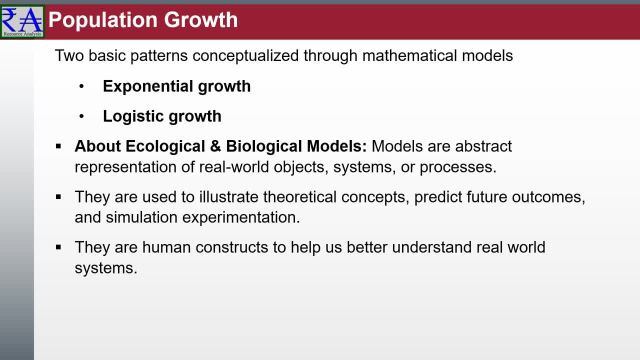 but that leads us to the habitat sustainability level, That ability of the population to exist at this level. It's a straight line. usually It never is in practice, though. We just model it that way because we want that apex number to show up somewhere. 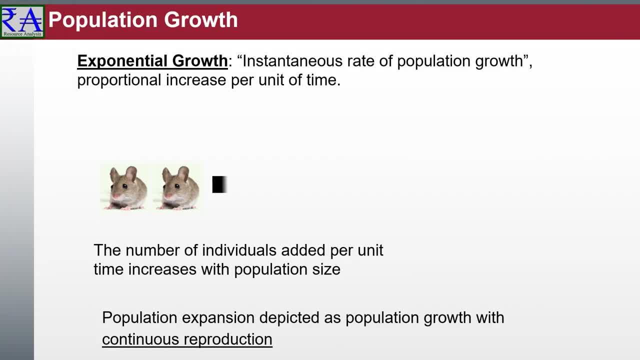 Really, what we're looking at is this idea of the mice: Two mice get together and what do they do? Yeah, they make four mice. And then those four mice get together and make 16. And 16 goes to 32.. Right, there we're doing a logistical growth. 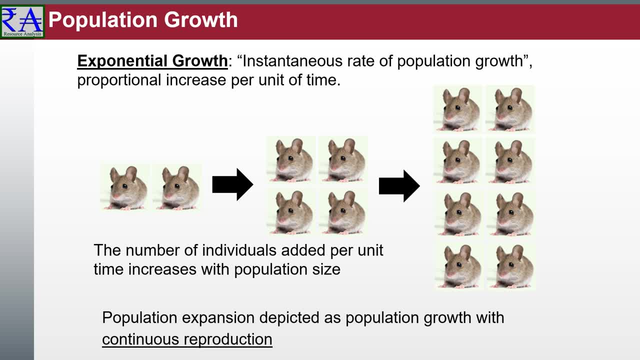 It's pretty constant rate of increase. It's not fluctuating too fast And it'll keep increasing forever. right, There's no limitation on the number of mice. Why not Echo Ding ding ding: Number of resources that can sustain the mice. 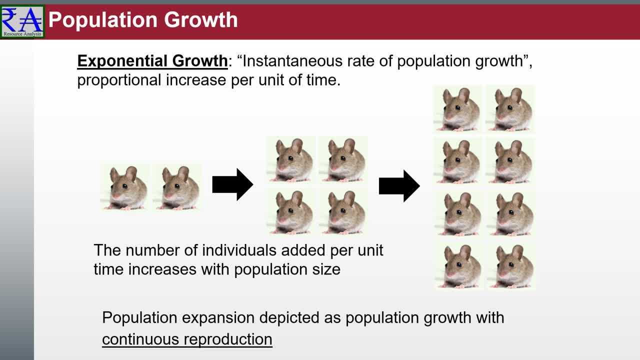 There's another limiting factor. Same thing that happened with the elk in the Olympic Peninsula. They were controlled and in equilibrium with their predator, the wolf. before we eradicated the wolves And then they started to increase at incredibly rapid numbers. It not only is the biggest elk in North America, 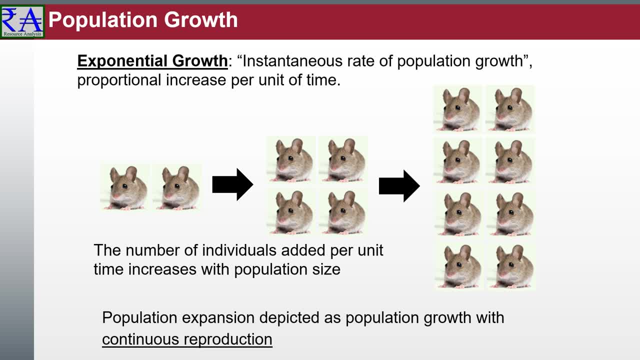 for body size, with the smallest antlers. it's also the most populated because it's the Olympic rainforest. There's a lot of vegetation there for them to crunch and munch on, But the limitation became their food and it became their space. Of course, it's a national park. 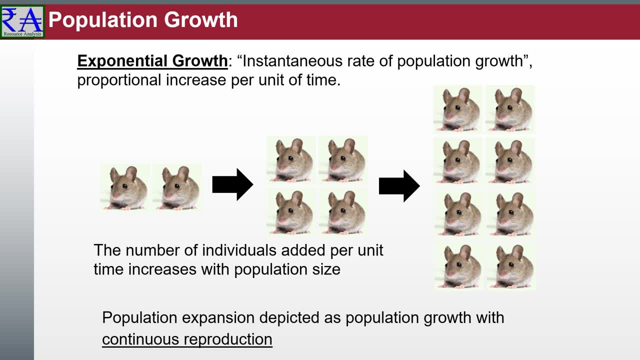 so nobody gets to go out there and hunt them, except the Native Americans who can go in there and hunt them. But really the number of animals taken that way, it's super small. You're talking about the impact of a couple of cougars. 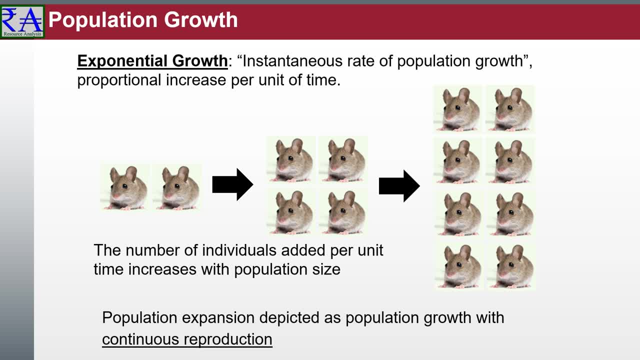 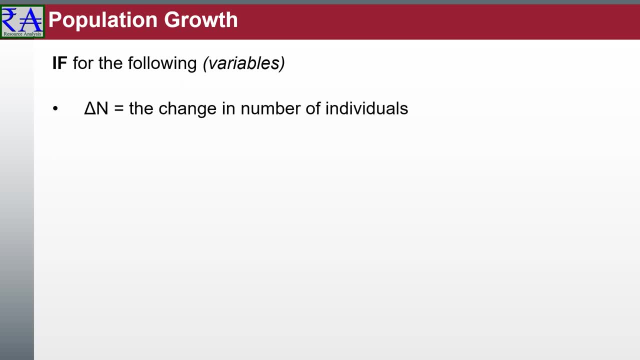 not a pack of wolves or a lot of pack of wolves. That limiting factor really drives it down. So we get a bunch of definitional numbers here. We talk about the delta N, That's the change in the number of individuals. We usually do this on a per capita basis. 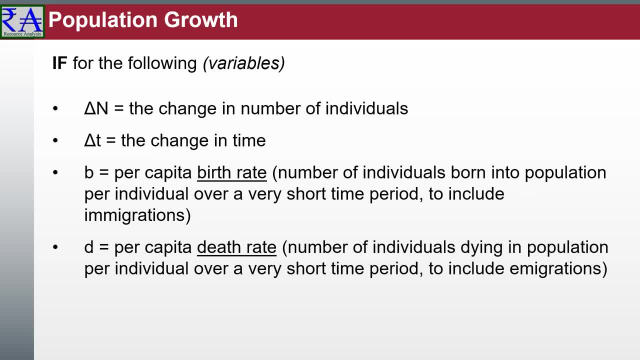 50 to 100 to 200 to 5.. You're just picking them out that way And the delta T is the change in time. How long does it take your population to respond to opportunities that are available to it? That's delta T. 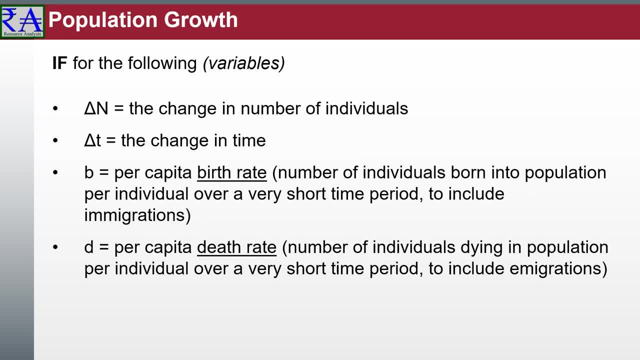 We're going to push it down to the beta and the delta. That's just your birth rate and your death rate And you can figure those out pretty fast to say: if your birth rate is high and your death rate is low, you've got the American population. 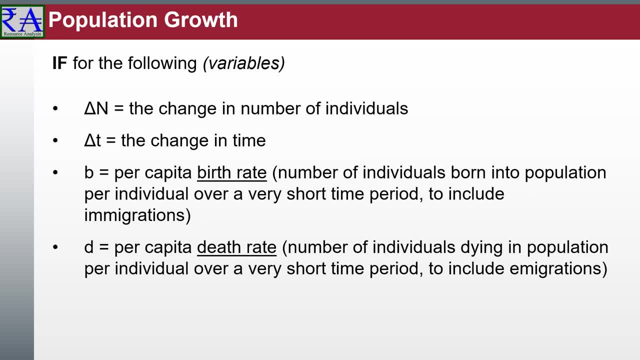 We've got a pretty high birth rate for a long time, a low death rate, and it's getting longer, longer. We've got a pretty high life expectancy That increases the population. We've all seen it. It happens day in and day out. 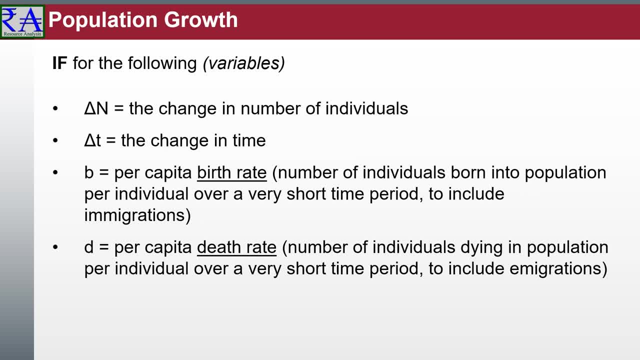 But really for natural resource ecology. we're going to tie up onto this over and over again because I do want to look at the populations that we're measuring. I talk a lot about the wolves and the elk and the deer, the cougars, but also I want to talk about the plants. 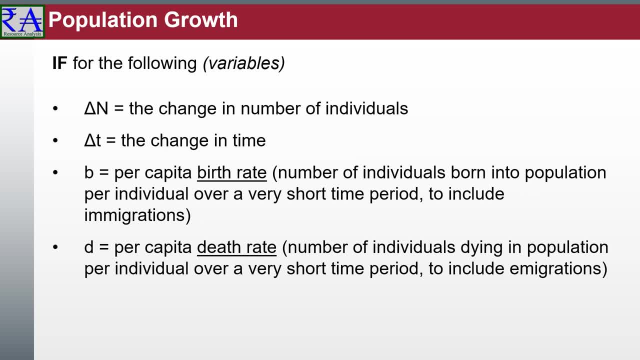 We can apply these same exact things to the tree species that grow in a forest, or to the shrubs, or to any other vegetative component that is competing for water, And it's going to increase the population. We've all seen it. It happens day in and day out. 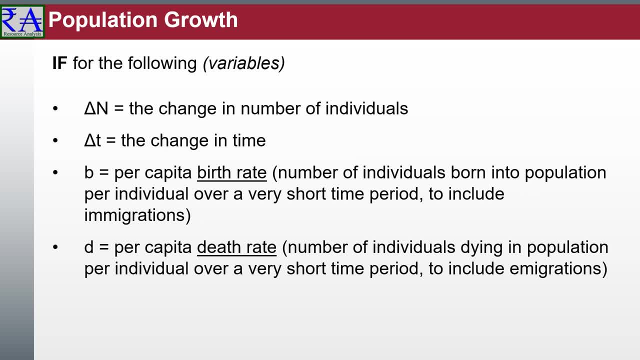 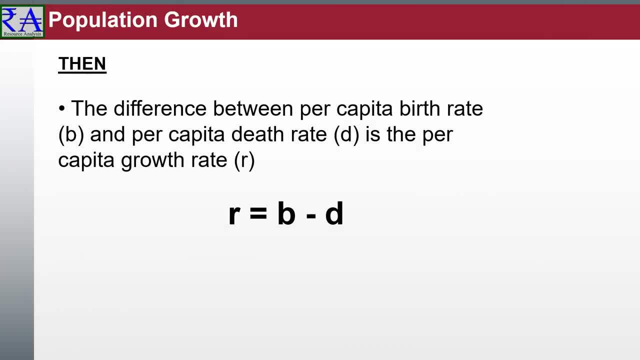 We're all seeing it And along the way it wants a lot of sunlight too. We're going to keep tying back into these, because that R- that is the rate of growth- it's going to be really dependent on that birth and death rate. 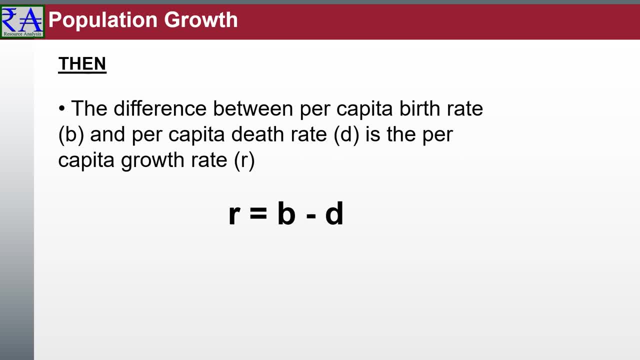 of that population we're looking to. Is it a constant thing? Not at all. That rate of change isn't constant. It's not constant with the human populations. It's not constant in the natural environment. Not a highly variable number in an equilibrium status. 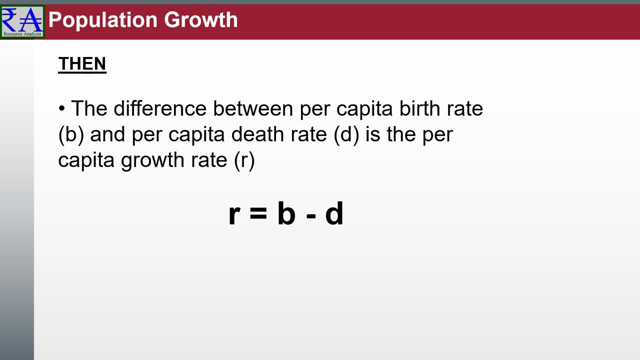 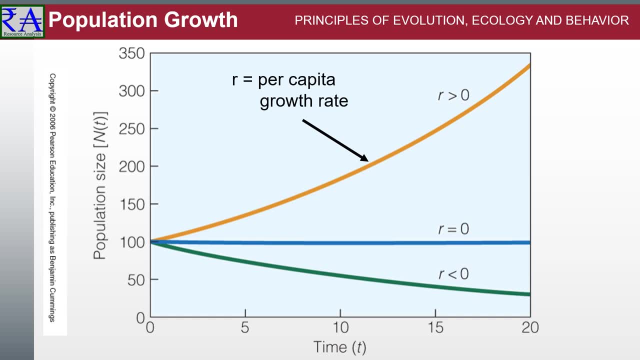 But as that population is growing or shrinking, you've hit to limitations at some different level. you're going to start to see these all take effect into different forms. One is these lines: Now, these are very, very simple lines, but that per capita growth rate greater than zero. 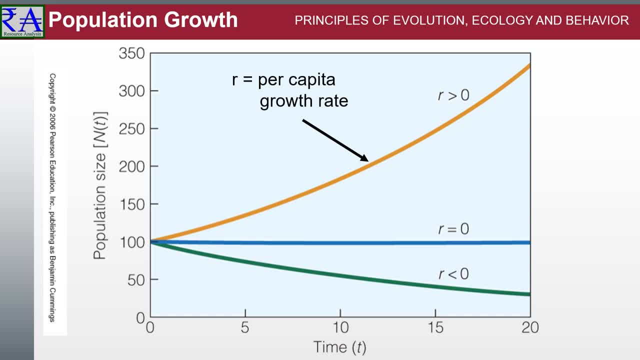 it's that orange line. it's increasing. it's going up. You got the horizontal line then going down at the bottom side. All of those graphs don't give us any good data. They're just a relationship for you to start keying in on. 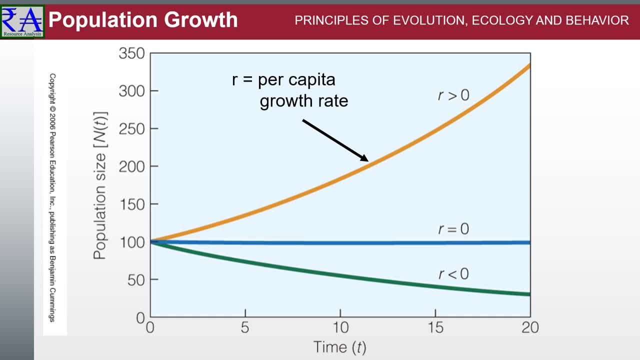 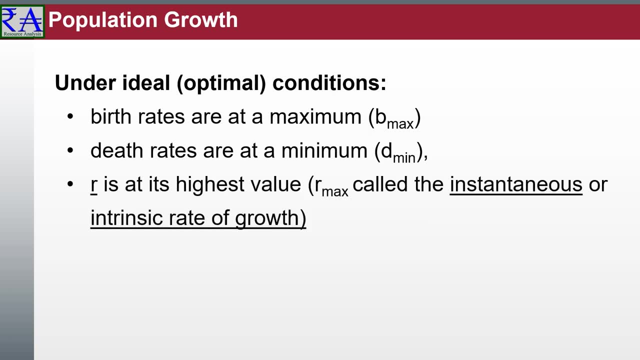 We are going to talk about. what is the potential of change, though? I'm going to look at that birth rate at its maximum. birth rate or the death rate at its minimum. Very few folks are dying. What's the minimum it can be? 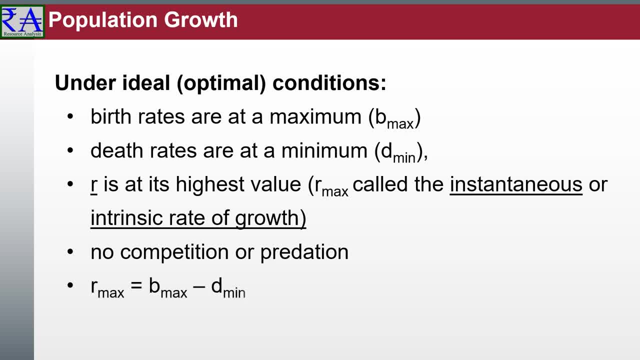 R, then, is going to be your highest maximum rate of change. That's a parameter, that's the sideboards that you put up on your schoolwork to say, hey, I've got to exist in this realm right here, which means I got to spend only two days on this class. 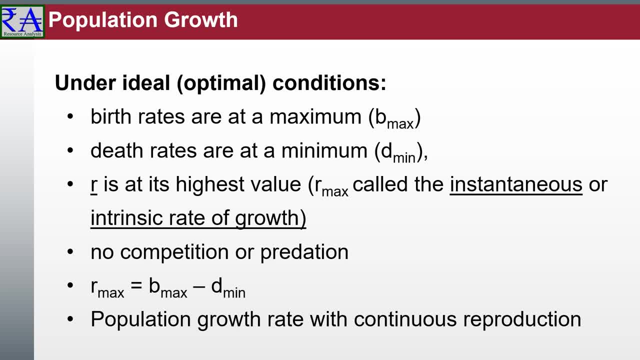 three days on that one and I'm done for the week. I haven't got any more days I can make Whatever you're going to put together, how you're going to piece it up, that same thing is happening with the populations on the graph here. 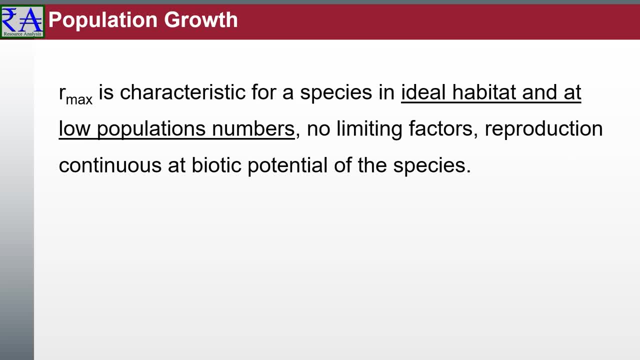 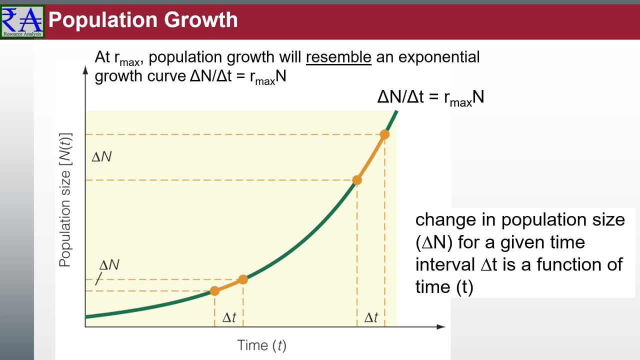 You want to try to figure out what are those parameters. As I look at this R max, this maximum rate of growth, what I really want you to focus on that line is a number of inflection points, That orange dot you see right down here. 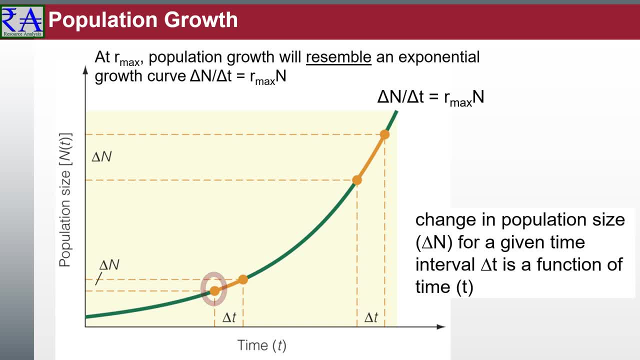 it's starting to build up as we are moving through that change in time. That's always going to be the delta time we look at What is the thing that's happening right now. Can we look at that rate of change Now? for everybody who had that calculus class: 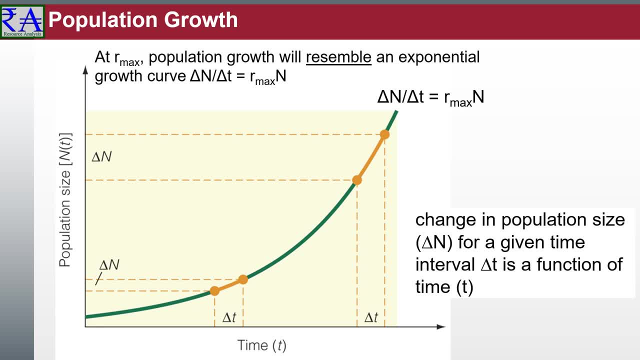 or maybe it was pre-algebra. maybe you've done some derivative work where you look at that rate of change and you take the first derivative of the rate of change, that delta t. you're going to try to express this as a marginal rate of change. 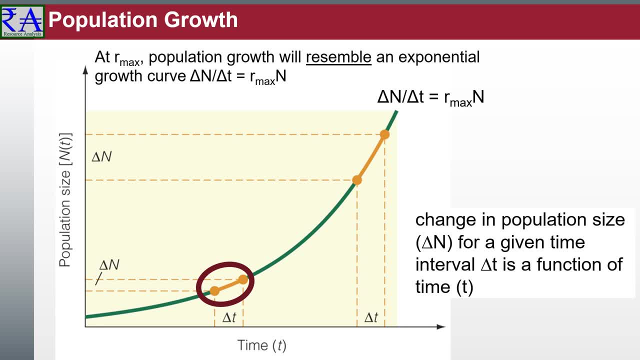 That inflection point that I show you in that first orange dot is that first rate of change, because that's where we went from increasing at an increasing rate. In other words, you're increasing the first step from one to ten. That's an increasing rate. 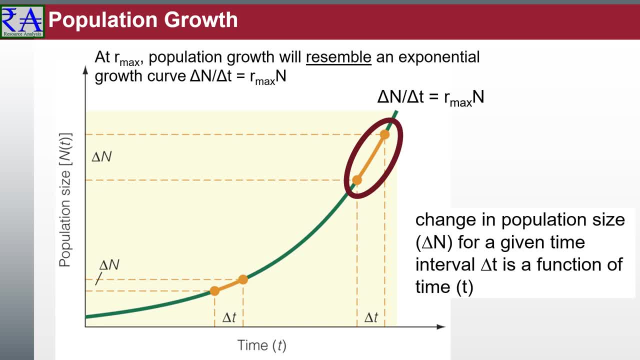 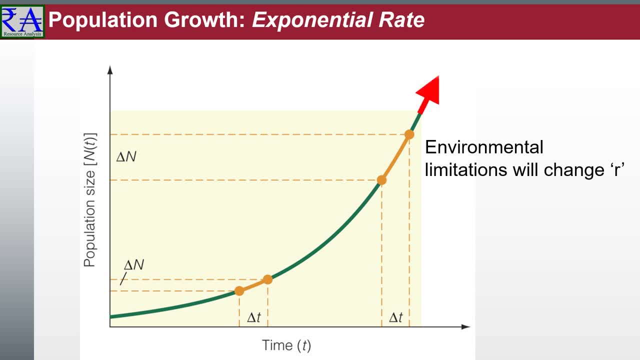 Ten to two hundred, Two hundred to a thousand. That's increasing at an increasing rate. This is continuous growth. This is the fallacy, because we know that even with the elk in the Olympic Peninsula, they have a limitation, Without the predator in place. 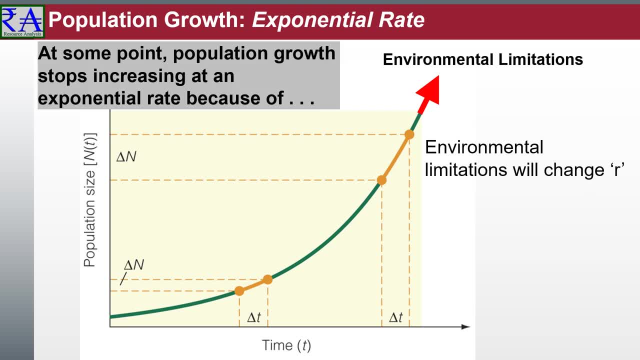 their limitation is food, it's space, it's a place to grow their young. That's the limitation for how many elk can exist on the Olympic National Park. Why are we going to move that around? I want to move it over here to look at that environmental limitations clause. 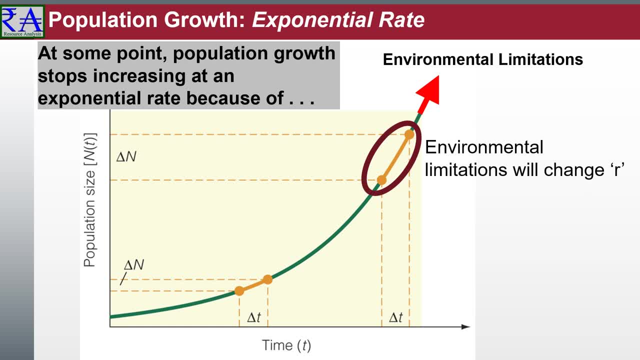 We talked about that, The idea that there's limited food, limited space, limited nutrition, but the food really derives all of that out, Because we're going to ask what is going to be the ultimate limitation? It's environmental limitations. What can the environment support? 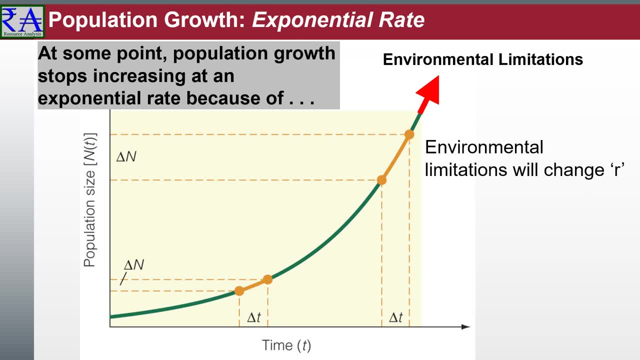 knowing that there's a load of different attributes that limit how the growth is controlled, whether it's the number of wolves or the space allowed? How about other species, other ungulates out there in the Olympic Peninsula that are competing with space against the elk? 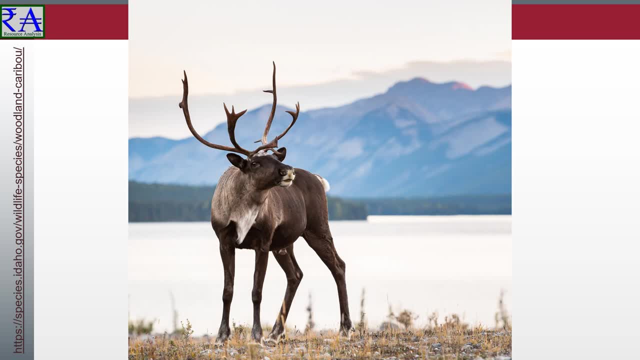 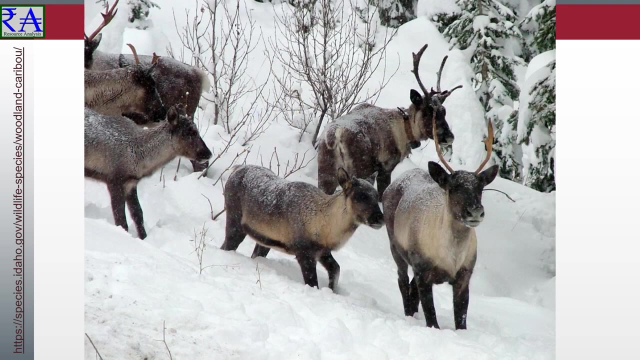 Do we have any caribou in Western Washington? Not a one. Do we have any caribou right here? Man, everybody's talking at once on that one Talk to me. Did everybody hear that There's some in Northeast Washington? 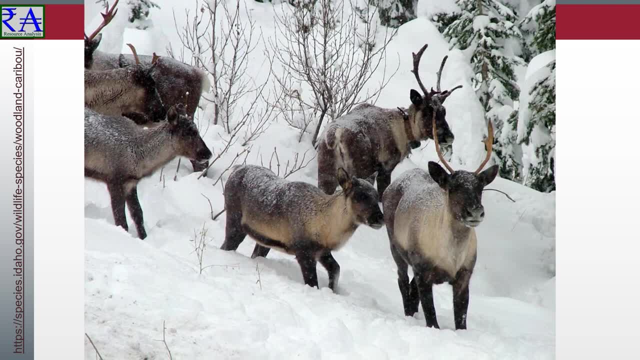 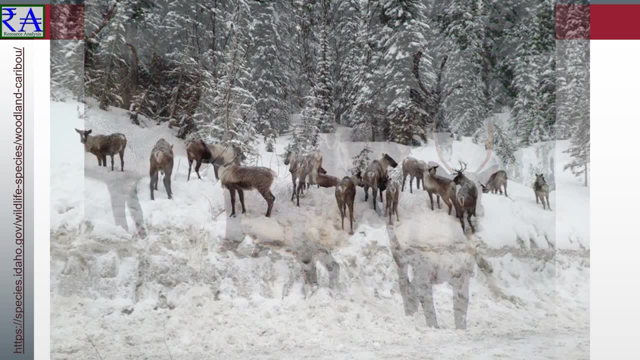 It came from Northern Idaho. How did that get there? Are caribou indigenous to Northern Idaho? No, but they have legs. Talk to me here. Did everybody hear that There's some in Northeast Washington? It came from Northern Idaho. 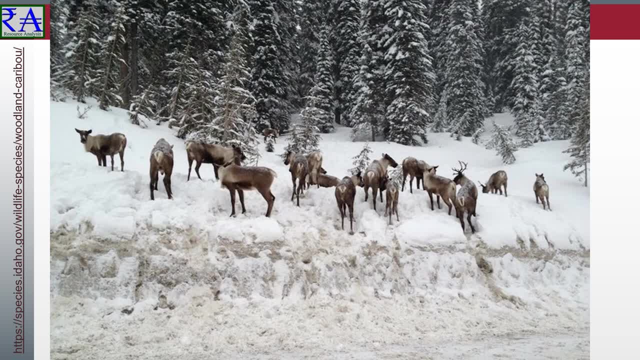 How did that get there? Are caribou indigenous to Northern Idaho? Maybe they were reintroduced or introduced artificially to that environment to see if they could thrive and survive? It's a very interesting one about caribou and I'll distract us very, very briefly with you. 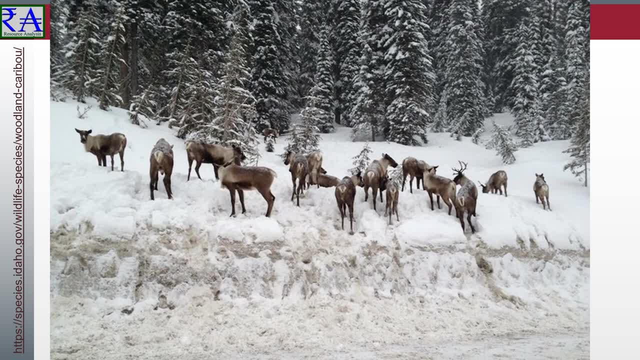 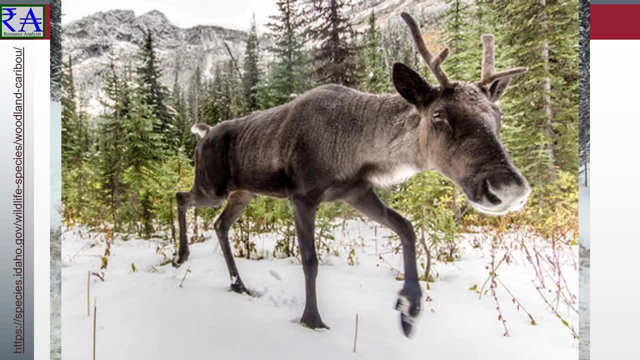 to say that the caribou in North Idaho were a huge topic for the Idaho Department of Fish and Game. They wanted to get out there and track them, make sure they could use telemetry. they can improve the habitat, give them everything they need. 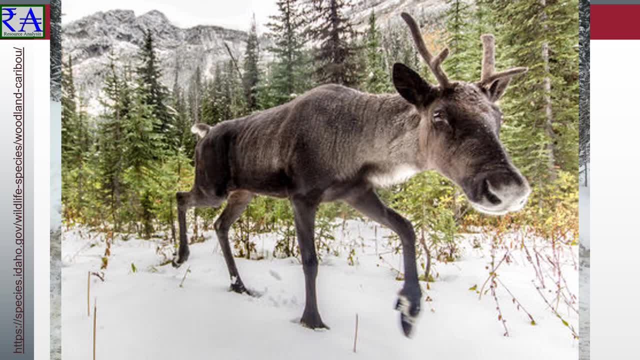 so they put collars on them. And these collars on these woodland caribou, when the bucks got into their rutting season, their necks swelled and they choked. Oh, slam the forehead, say oops, The movement of those caribou. they came out of Canada. 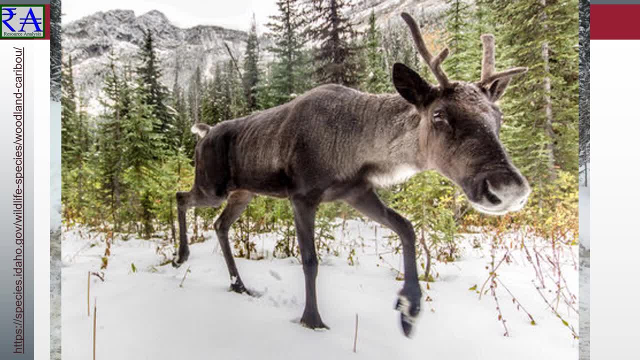 I'm going to talk about metapopulations coming up on Friday, That metapopulation that spread into Idaho, that then was spreading into Northeast Washington. are they going to fill it up? They sure could. That was one of the cases of humans. 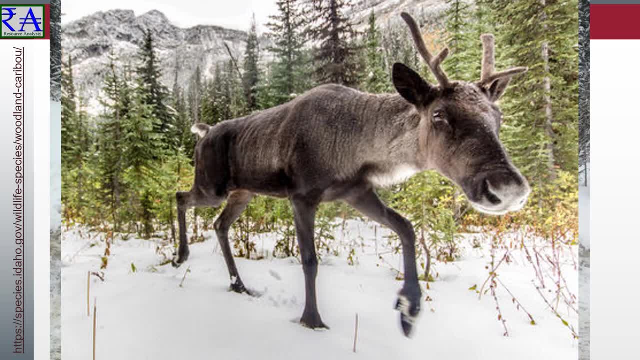 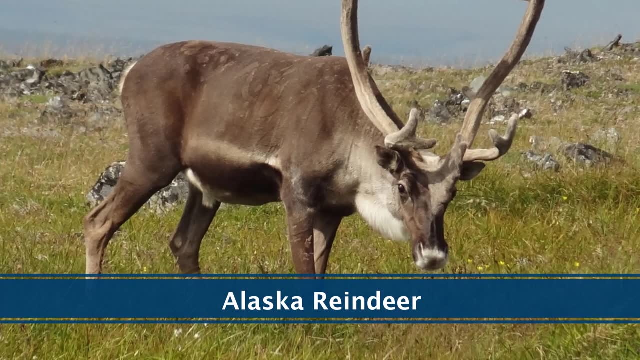 having a high interest in wanting to track these population numbers of a species, woodland caribou. But we're going to look at the environmental limitations. And now another environmental group: Alaskan reindeer. Reindeer is the name that the Europeans gave to caribou. 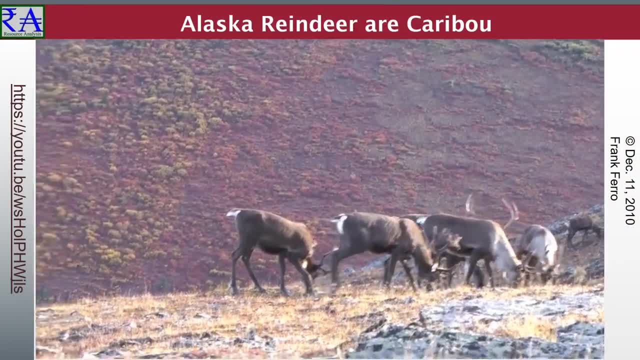 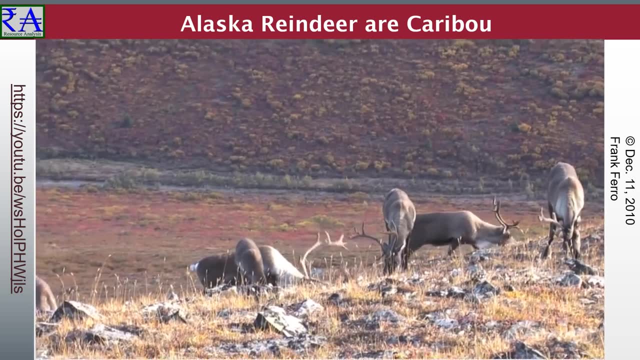 The caribou are indigenous to Alaska. there's no question about that. But right here you can see what kind of habitat they live on Those caribou. they are not in the timber. those caribou- at least Our woodland caribou- are in the forest lands. 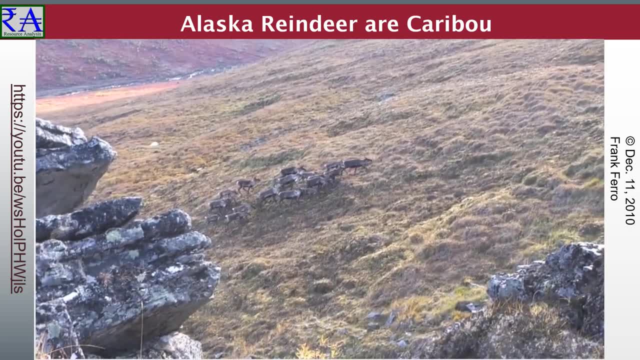 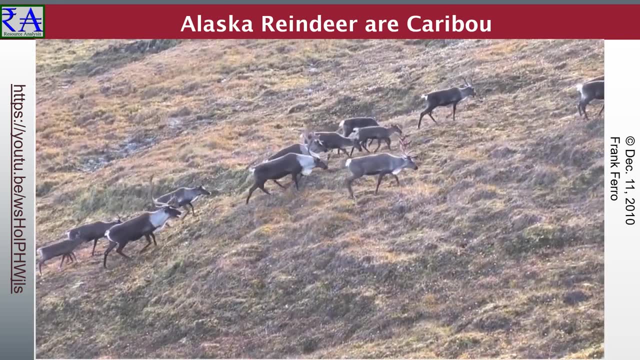 but right here they're on grasslands. They're in that countryside within Alaska, and big, big numbers, Huge herds having a good, sustainable life. They're also a migratory animal, like the elk are, but they're a different size animal. 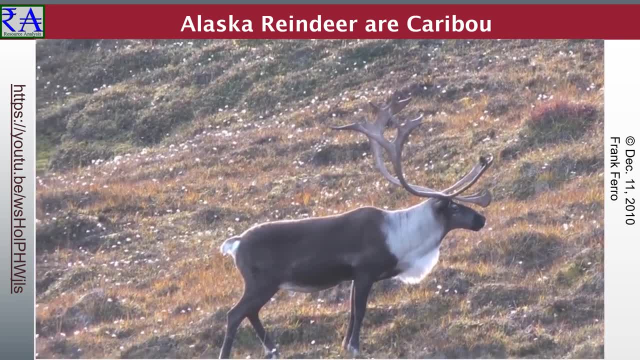 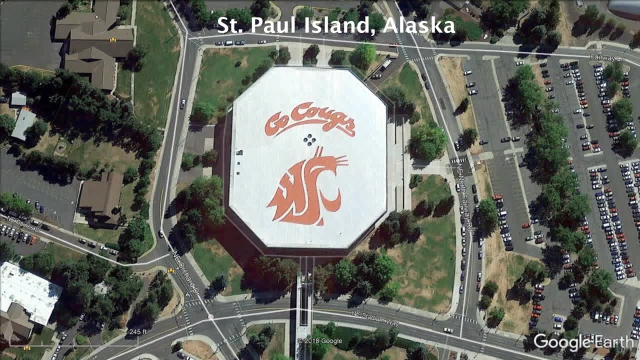 These are super big, The ones we have right here in Washington and Idaho. they're woodland caribou. They're about the size of our deer. So what I'm going to do now is take you to St Paul, Alaska. We looked at the Bering Straits before, didn't we? 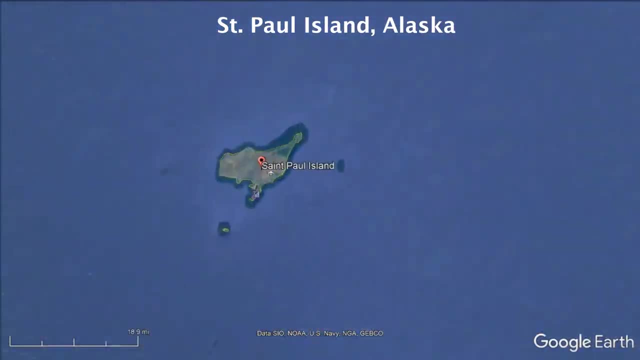 So much water was locked up in ice. Well, we get out there to this Bering Sea area and there's St Paul Island. This island- it's not the biggest thing in the world, Well, 12 miles long. It's got great habitat and the idea came up. 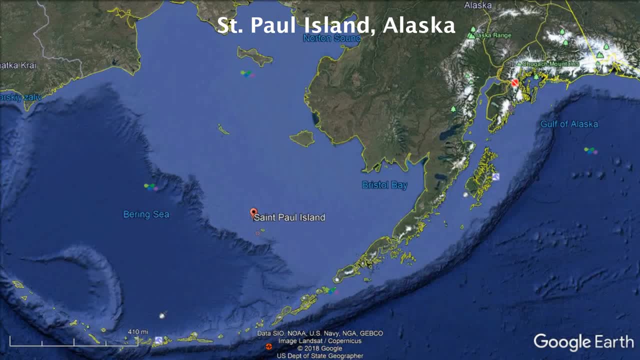 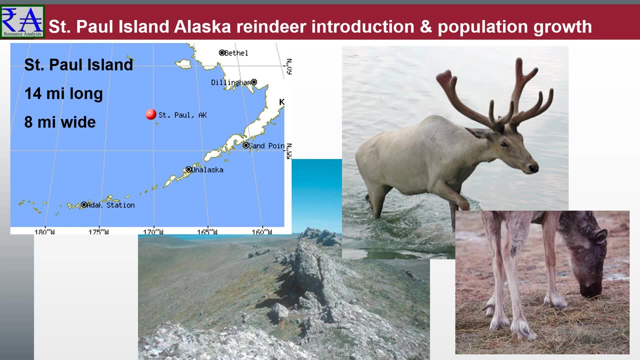 how about we put some reindeer out there? There's no predator, There's nothing going to knock them down. Let me take the sideline step before I get too deep, because I have a brother-in-law. sister's husband is a commercial fisherman. 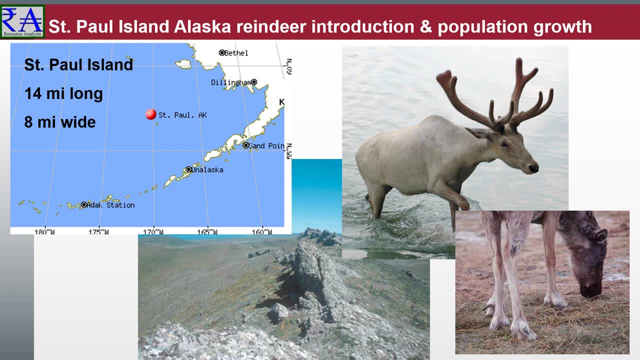 He grew up in western Washington with me, So Murray does the deep-sea fishing in the Bering Straits right there He does crab, He does salmon, He does halibut, a lot of cod. But he stops at St Paul Island on his way out every season in the fall. 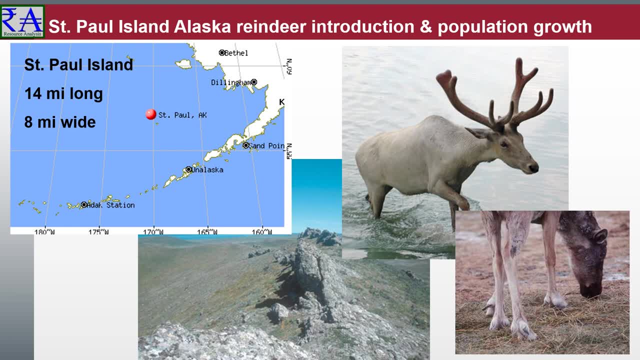 because his crew wants to go hunting for caribou And it's a special hunt because there's a lot of animals. Well, here's how that lot of animals came about: This St Paul Island- it's 14 miles long. 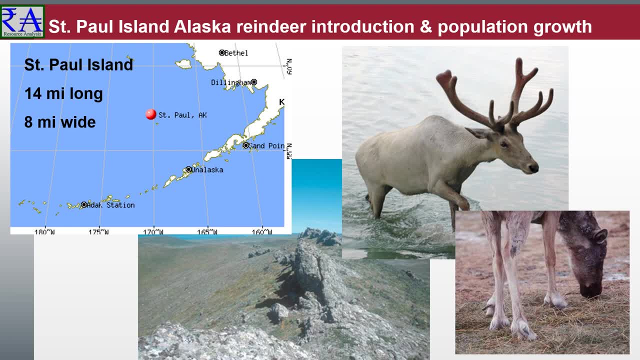 I think I said 11,, 8 miles wide. It's a real rocky, barren land. It's in the middle of the sea. Can the caribou naturally swim out there? Nope, ain't going to do it. So they got transplanted and put out free to run in that environment. 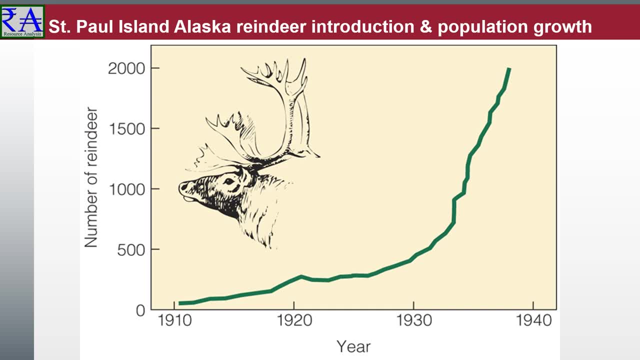 And here's what happened. Their numbers increased super fast, Exponentially grew. They had no problem surviving Lots of food they'd never been browsed on before. All that grass, the mosses, the things that the caribou loved to chew on. 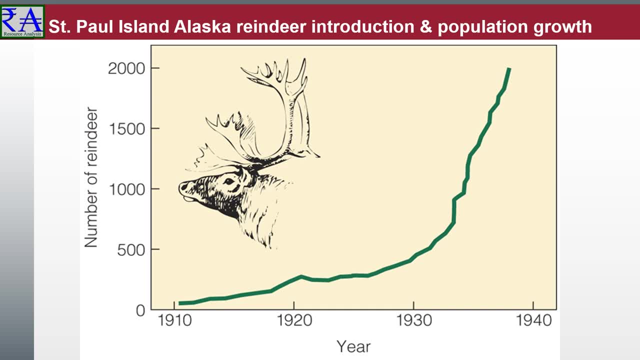 they were plentiful, Their numbers skyrocketed. Could it keep that skyrocket going forever? Well, one side is, they did have to introduce a predator pretty quick, because this happened around 1910.. They dropped those animals out there- about 25 critters. 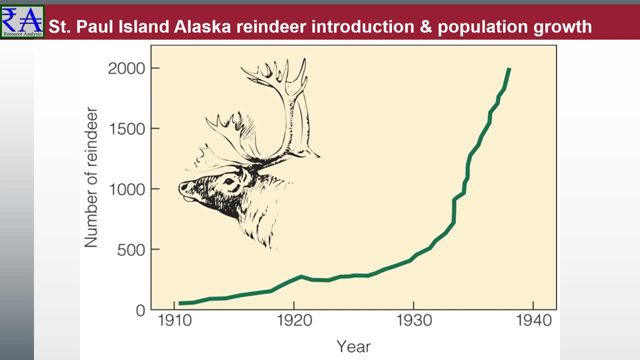 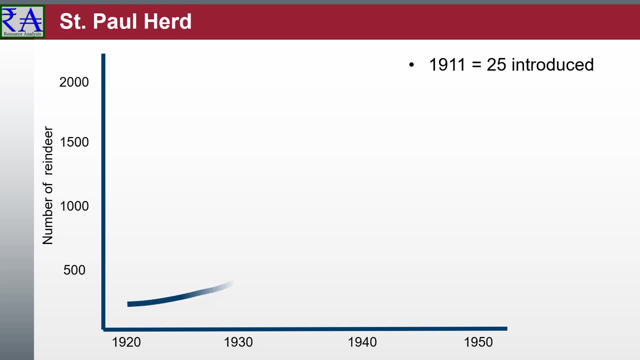 and let them breed and reproduce. very fast You can see their numbers increasing. This is the kind of population growth that we talk about. And then that population, it hit its apex. It was a peak followed by a trough. That trough is because the animals overpopulation. They took out the food. They filled up the space, But it was the food that was the most limiting. They had to have fresh water to drink. They had to have the grasses to eat. All of a sudden, the animals became sick. They became disease infested. They dropped all the way down to what you see right here. They got down to eight by 1950.. We're super smart as a human population, aren't we? We can do anything to the critters that we manage. 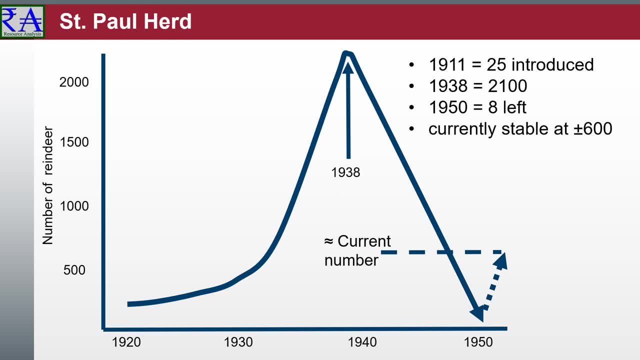 We can eradicate the wolves. We can put an unthreatened caribou. a little tiny herd out there grows up to those 2,000 numbers. They trough, They tank And now they're being sustained. And the only way that they could get that sustainable number. 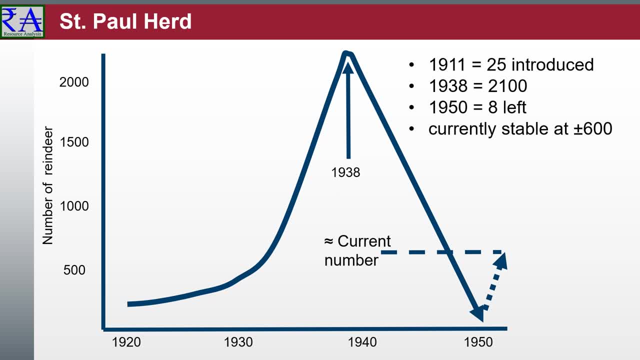 to maintain about 600 critters is by introducing a predator known as humans with their rifles And crews like my brother Murray's. come out there and do a special hunt of caribou on this island, A little tiny island, real high success. 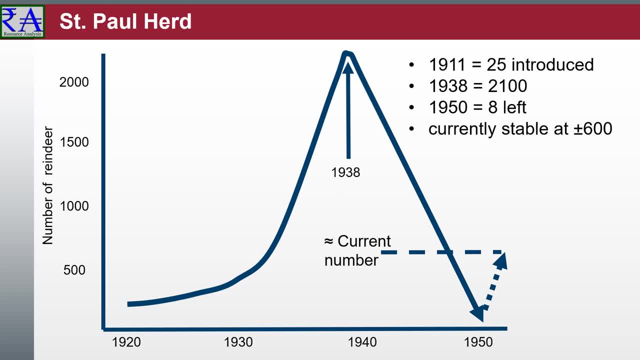 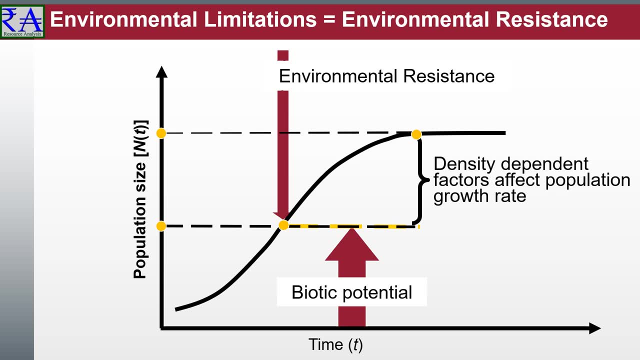 That's the only way they can keep their numbers under control. So how really do we hit this biotic potential? then, Going back to that island example or any of the other examples, this is that inflection point that I talk about. This right here is going to give you that hit of the inflection point. 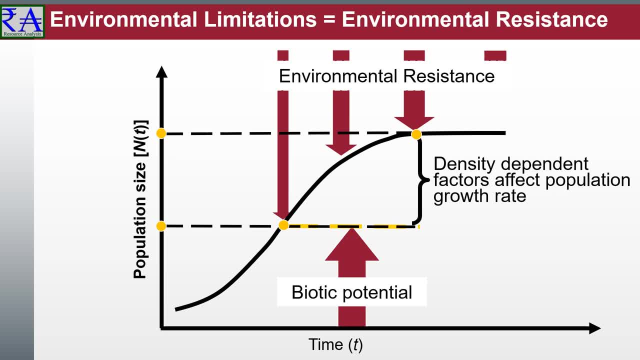 If you're doing that derivative of your equation. it's talking about the potential of the site to sustainably support that population in that environment And it's very specific, environment by environment, That density dependency. it's tying back to all the things I keep reiterating. 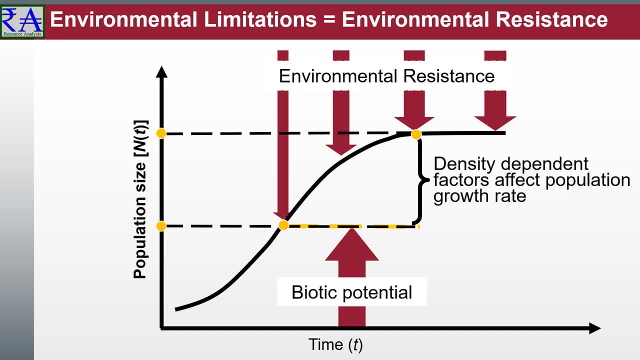 their space, their food, their ability to live their life cycle. That is going to determine, species by species and environment by environment. what the potential is- That's really what I want you all to be able to do- is to have a feeling as you look at that ecosystem. 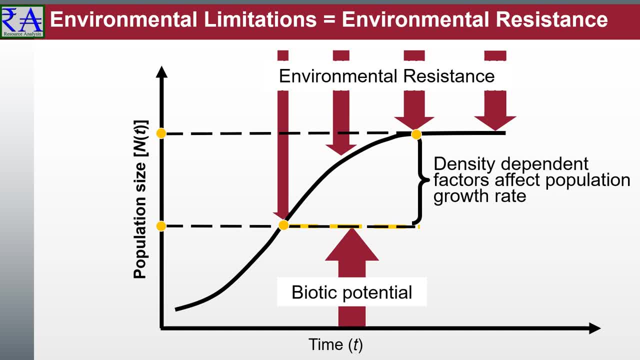 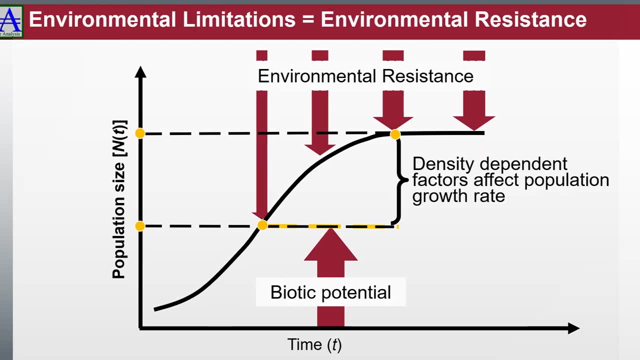 how it can support all the species that are there today. the predators, that whole intermix from the apex predator down to the other predators, down to the consumers, those primary consumers and secondary consumers, right down to your initial primary consumers, primary producer plants. 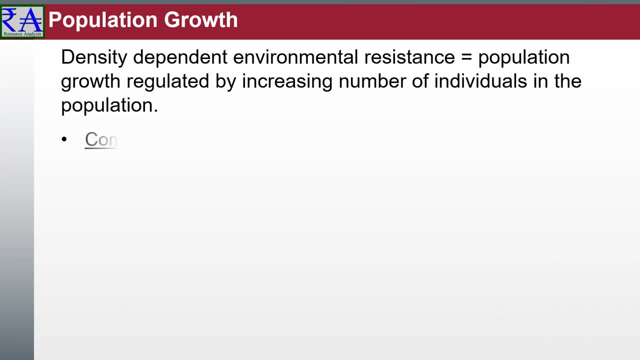 Interdependency. That's what I want you to really understand: that that adaptive response is going to deal with how that population has a social structure, And there's totally a social structure to a lot of this. It's what I talked about early on with the birds. 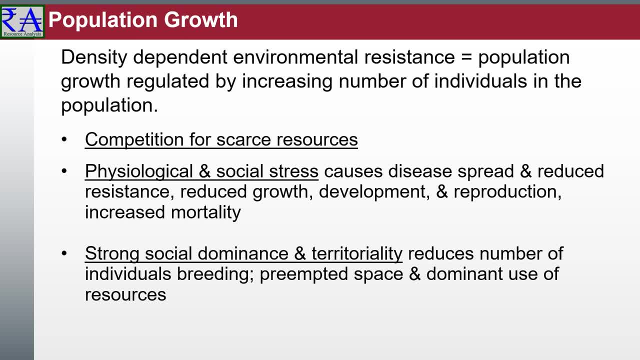 They get kicked out of the nest, They put out their wings and they soar. It's not immediate, They're going to learn it, But they have the intuition. They have the adaptive trait that was passed on from generation to generation And the reason all those elk are going to follow. 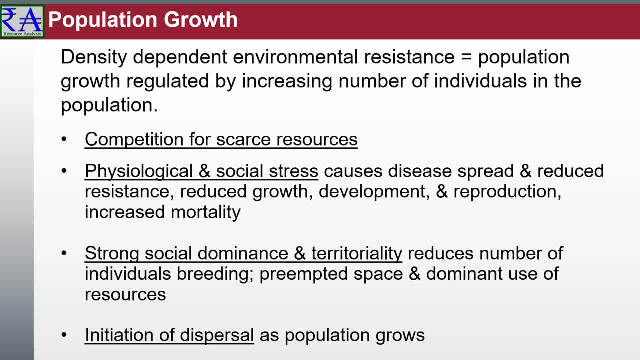 the lead cow and the lead bull, as they do their migration. that is bred into their adaptive traits, That is their social structure. It works pretty well because we can see all kinds of interactions, whatever species you're talking about. I talk a lot about the trees. 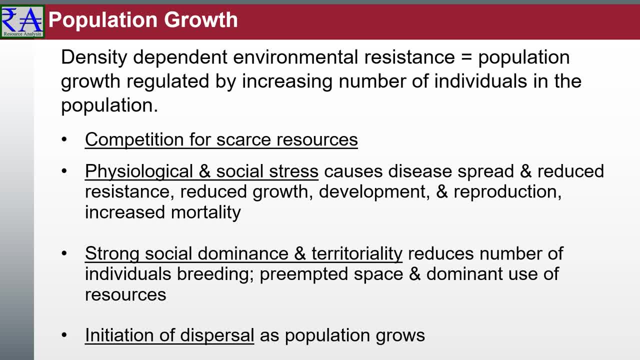 I talk about the economy too, But really what I'm focusing here is to say: it can be the trees, it can be the shrubs, it could be the salmon, the elk, the wolves, anything else you have for a population group. 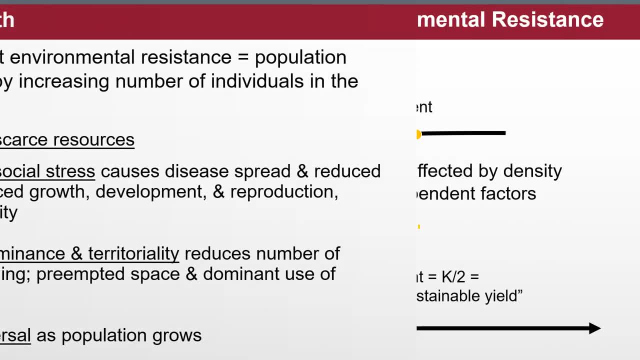 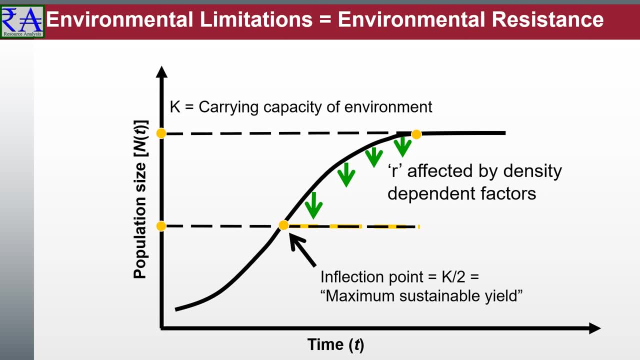 How are they going to respond And what are the interconnections? To look at the inflection point, that K divided by 2, to understand that is an important interaction right there If you can recognize where that hits, as it's hitting as it's growing. 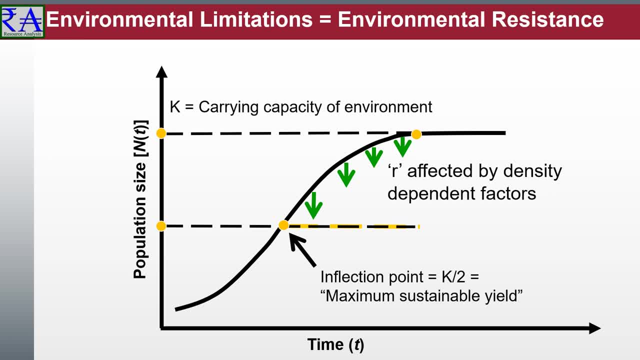 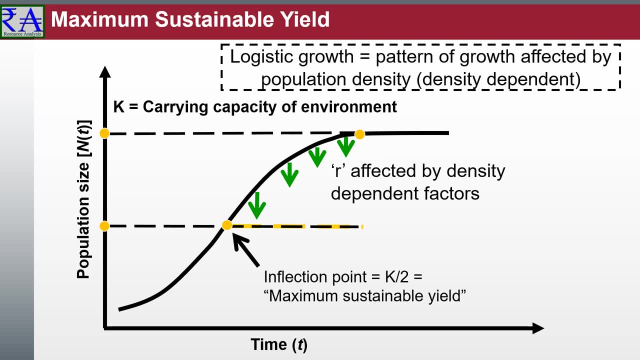 you're going to make a lot of predictions about where that apex carrying capacity is. It's that gray matter between your heads, folks. I always want you to be able to put that feeling of where is a legitimate number of your prediction that things are going to. 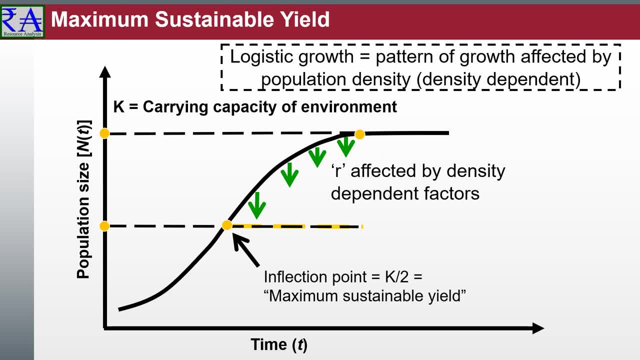 go here or they're going to go there. That's the kind of graph you're going to make. You're going to look at your populations and try to do that modeling to stretch them out, to say where is that logistic growth pattern? It is this idea of filling the barrel with water. 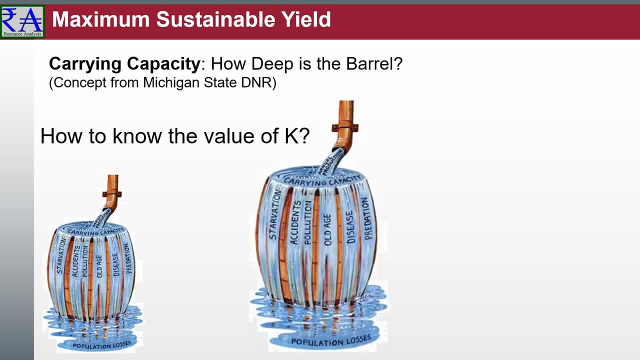 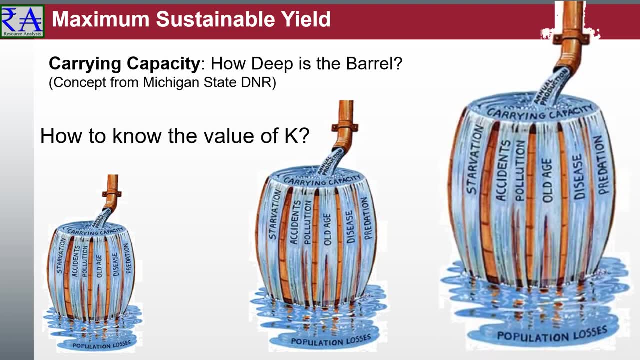 It's got a carrying capacity. You keep filling it up. pretty soon it's going to overflow And the big question becomes: how big is your barrel? If I'm talking about the Olympic Peninsula, my barrel is how many critters it can support. 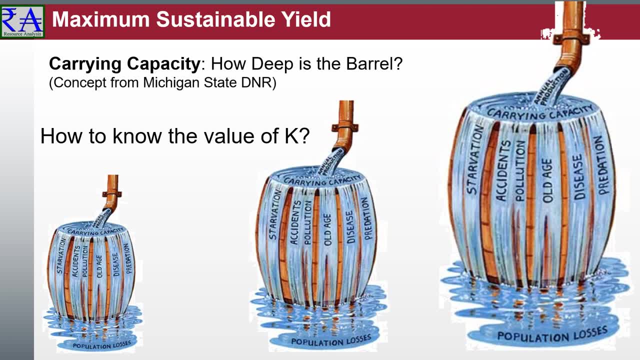 based on those otter-troph plants that are giving the nutrition to the animals that feed on it. Even when you take out the wolves, there still is an apex number of elk that can live there because they've got to have the food to eat. 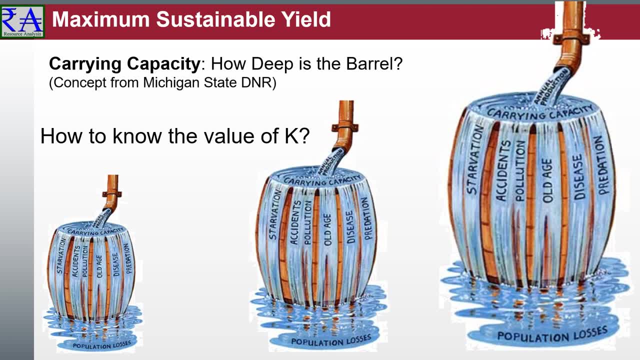 This all of a sudden makes all of the wildlife managers in the room very cautious of the idea that you also have to be a plant ecologist. You've got to figure out how many plants can grow out there, What's their dispersal, What's their timing. 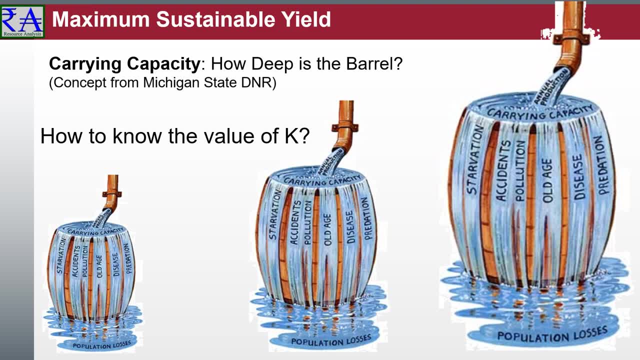 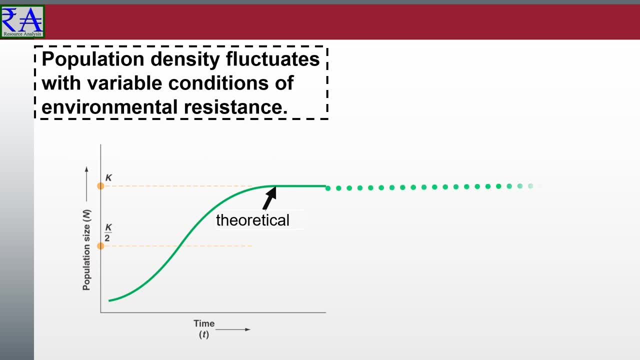 It's not just having all the great plants. in the spring, when the water is plentiful and the sun is high, It's getting cold. Nothing's growing green. We've got to have plant vegetation for the herbivores to eat If they can't eat. 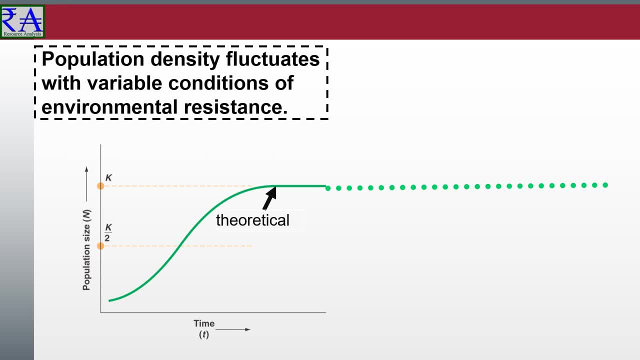 they're going to die this winter, So they find other things to feed on. What is their fat reserves? What is their bank account of energy in their body? As we look at this nice horizontal line, really it looks like this: A bunch of little peaks, of a bunch of troughs. 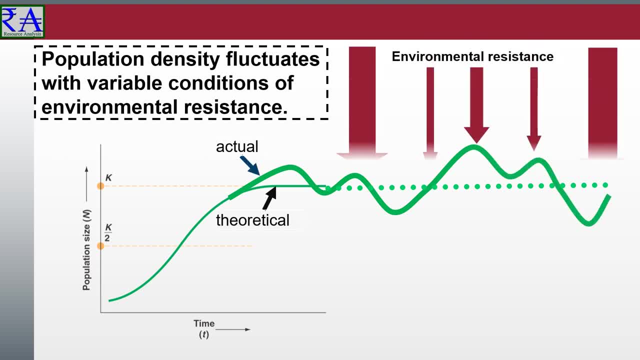 And in economics I refer to those as random noise shocks. That's exactly the same tradition that we see on these population number changes. There's peaks, There's troughs, And they all come about because something maybe we didn't model in our projection of what the population can grow to. 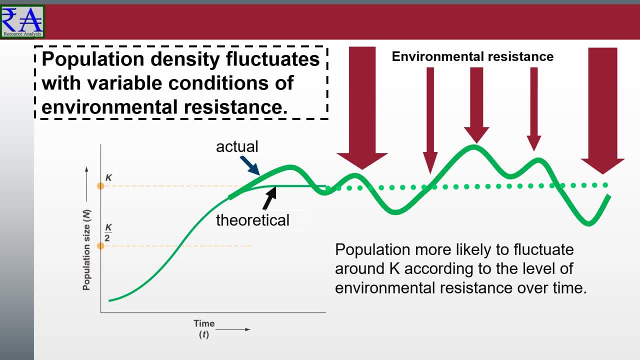 We may not have picked up that little tidbit. Be cautious of these. Just know they're going to happen. Those fluctuations are going to be a part of the carrying capacity of that cave for that site, on every site you look at. Let's step into a couple of examples. 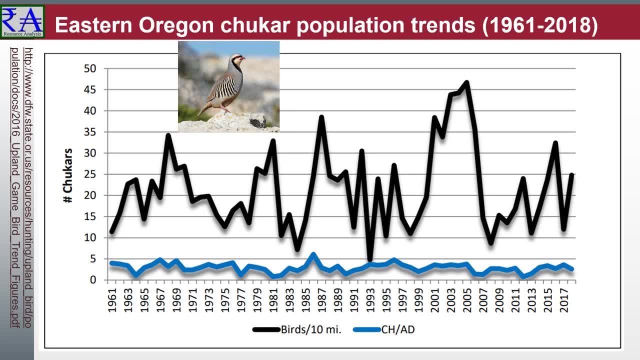 We'll even look at partridges here and different ways that we measure how that moving average really looks. That moving average is the blue line down below. We're talking about the number of chicks per adults going up, going down. That's a running average. 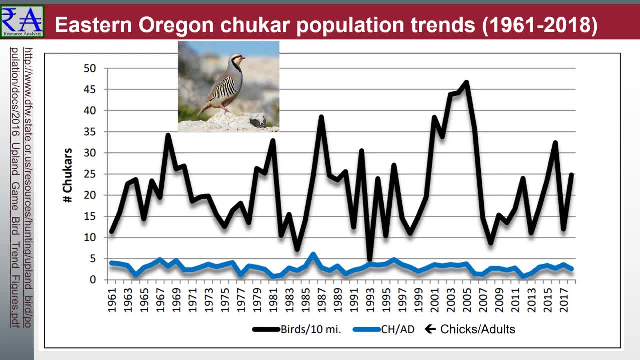 And you see a peak and a trough. Look at the big number or the big line in black. It's talking about how many are total out there. By looking at the chick-adult ratio we can get some predictions on what's going to happen eventually. 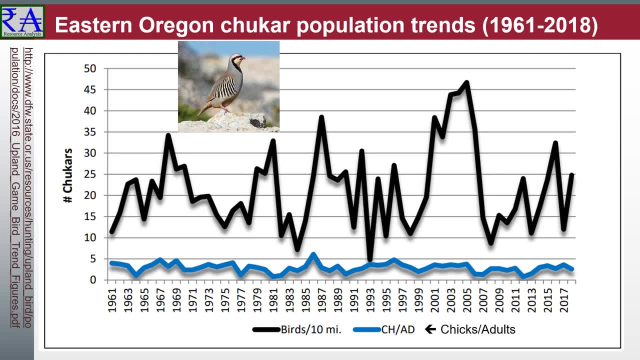 for those big numbers. You see the peaks and they trough off again. Generally, those are a combination of two things: Predators being more successful and it's the food being overeaten. All of a sudden, a limitation- The partridge numbers drop. 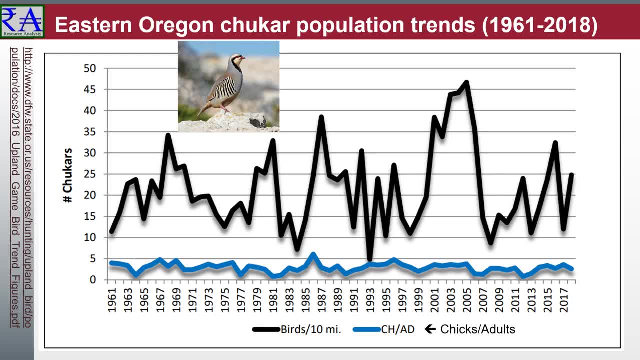 Drop like a rock because they can't support that many in that environment. It's that carrying capacity, That carrying capacity. we're going to show it all the time and everybody does. It's that peak and the trough across the top, The random noise that you see on that graph. 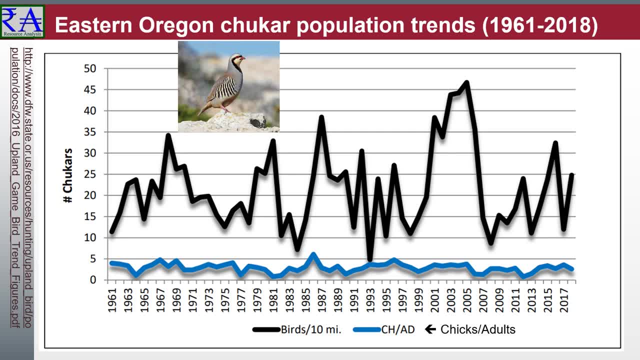 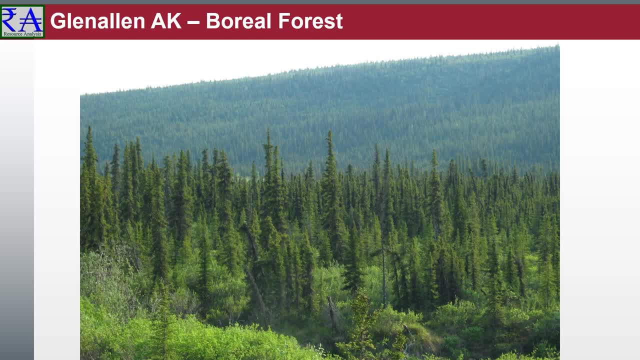 That to me is the carrying capacity of the site. And let's go back up to last, slide Back up to Alaska, into the boreal forest, Back to our good friend the bunny, The hare and the lynx. You'll watch that video. 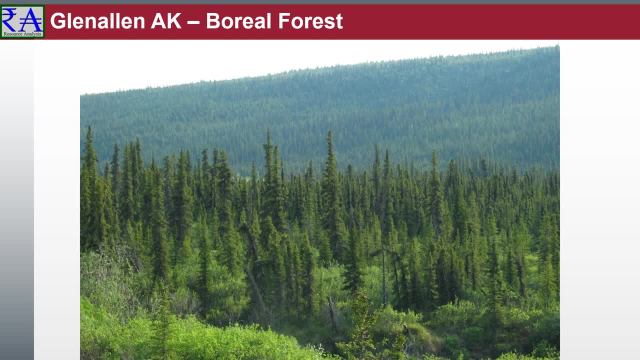 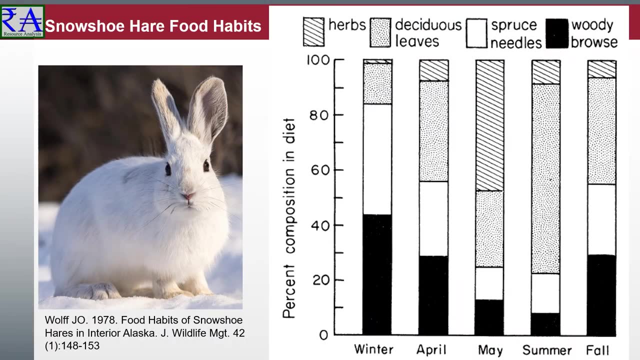 You saw that interaction And the big thing about the lynx is not wanting to spend more energy on capturing that little hare than his nutrition is worth. That lynx is an economist. He knows totally about the marginal gain of trying to spend money or energy. 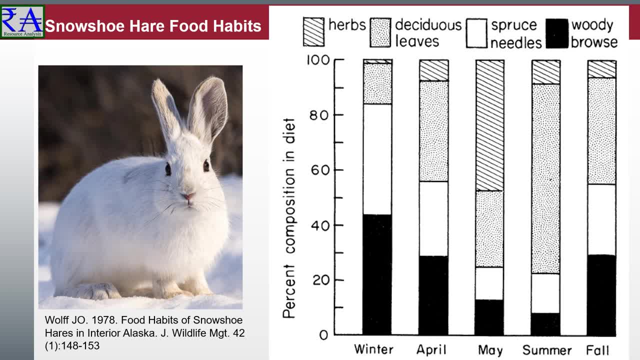 to get that little benefit of eating the bunny. It's a hare, It's not a bunny. Dr Bill's trying to make some humor out of this. You've got to look at what is that hare eating now? This is the carrying capacity of the site. 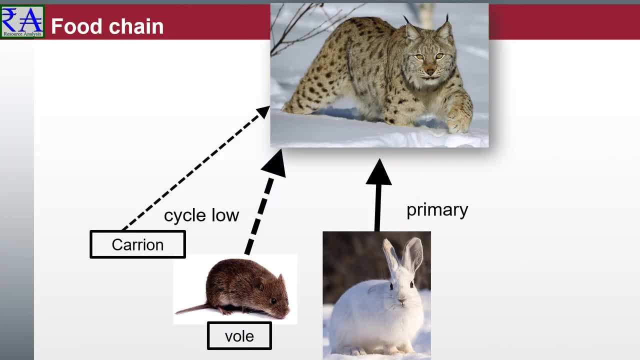 not just that one snapshot in time, but going across the entire seasonality of the food sources. Sometimes it's eating on that green grass. It's eating on the green brush, the herbs, pine cones, woody materials in the brush that it was eating on. 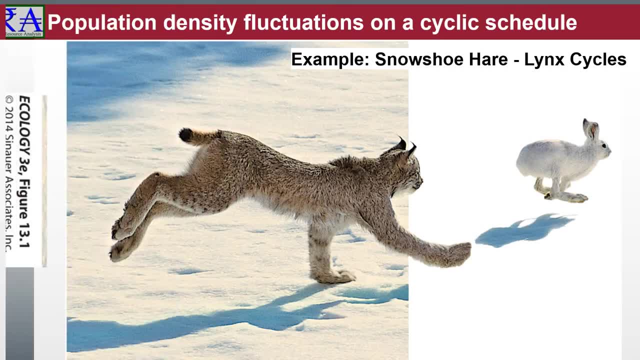 Oh, its numbers aren't going to necessarily drop. it. It's not going to be so vital as to be a growth in the time of the population. That's why a lot of times their breeding seasons, for hares at least, are tied in to the growth seasons.